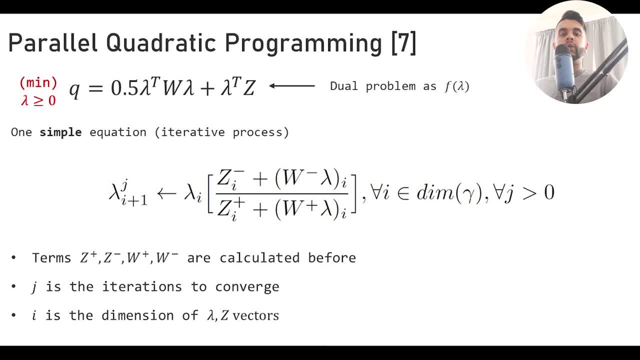 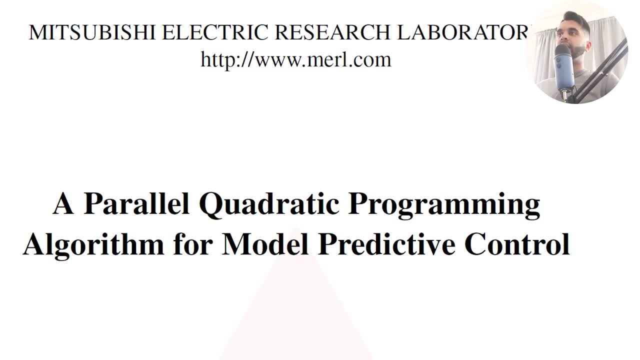 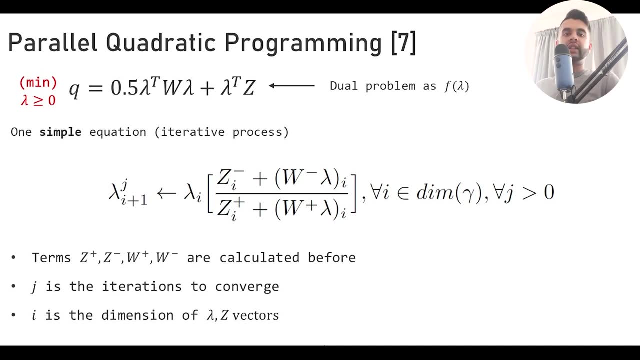 And this is how you activate a solver. We'll be looking at the PQP algorithm. This was invented at Mitsubishi Electric Research Labs, or MERL. This is a very high performance R&D facility in the USA which does a lot of work in autonomy controls and so on. So now let's begin the simulink example. 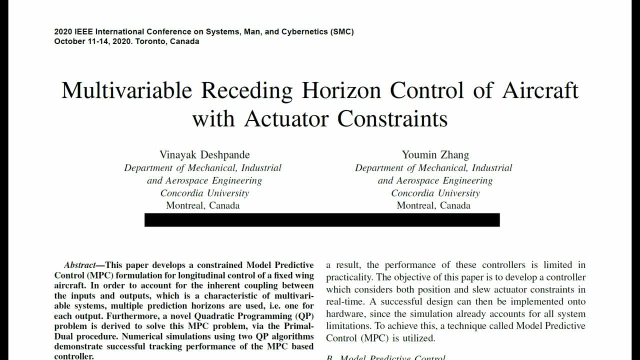 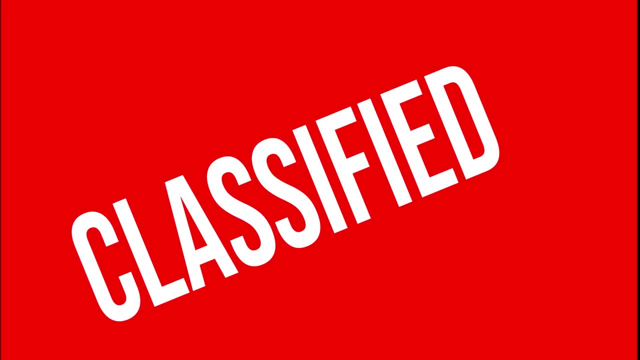 So this paper, I had the opportunity to publish it on my website, which is wwwmitsubishicom, during my master's degree at Concordia. it talks about MPC and optimization. I will directly skip to the optimization section because for the MPC, that will be. 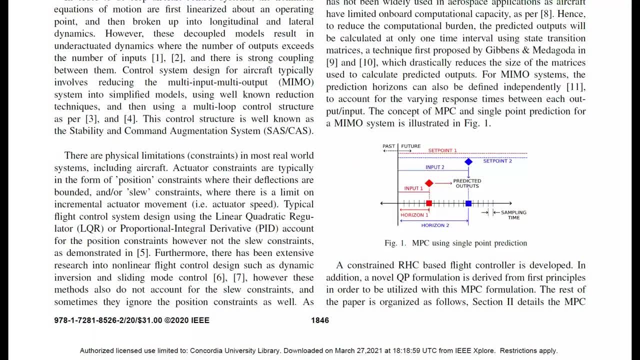 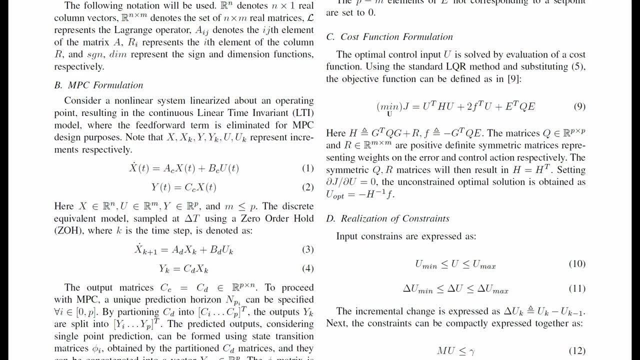 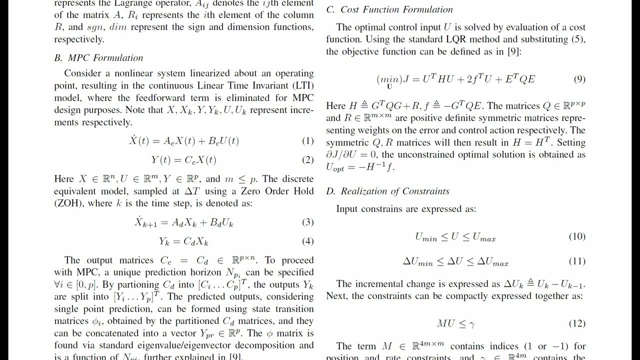 covered in a different video. so whenever you optimize something, you have to use a cost function, you have to develop this yourself and you also need constraints- right, because the whole point of optimization is mostly when you have a constraint on something and want to make sure that it does not exceed that value. 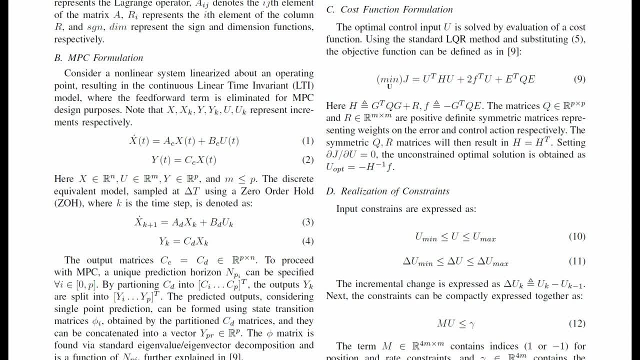 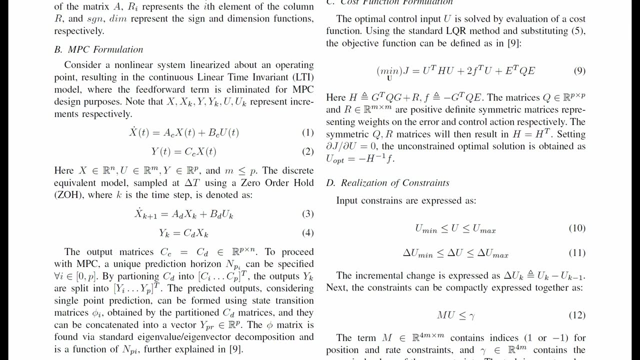 so in this case we have input constraints, the inputs are between minimum and maximum, and also on the Delta input. so Delta U and Delta U max, which is between each time step. so from equations 9 & 12 you have to use something called the duality principle to get these equations here. 13 to 15 you 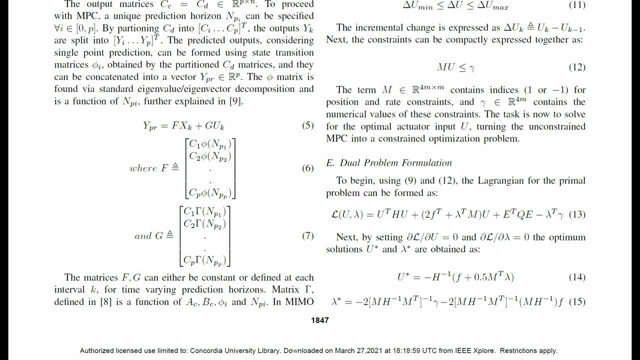 have to differentiate the cost function with respect to the optimization variable. so in this case U is the optimization variable, lambda is the Lagrange multiplier. so this is very common principles in optimization. you have the off the variable and the multiplier and you have to solve for the optimal values. so this takes into account the constraints and 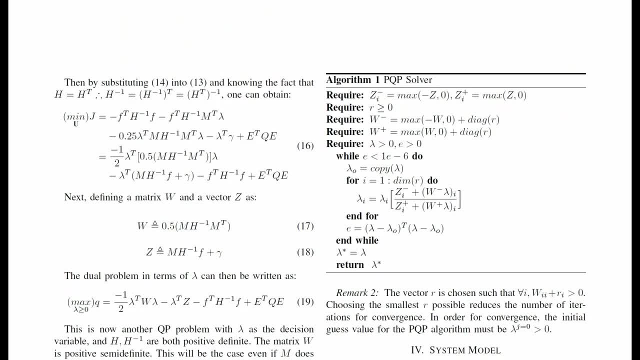 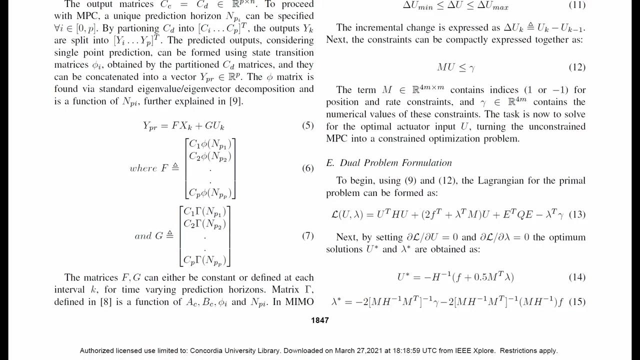 for our optimization algorithm, you have to define two terms: W and Z. now, W and Z can be defined before, so they are based on your system model, which I will get into more details in the future. so for now, just make sure that you have W and Z, along with M and gamma here. so these terms have to be defined before when you 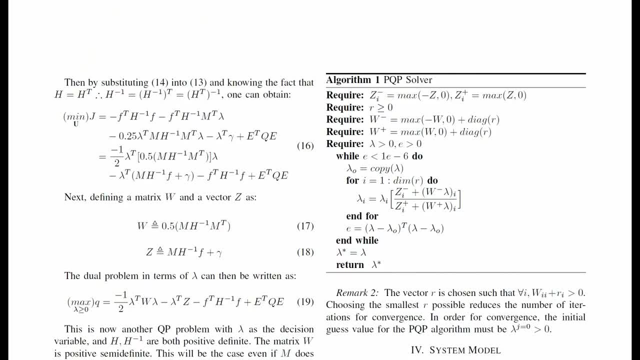 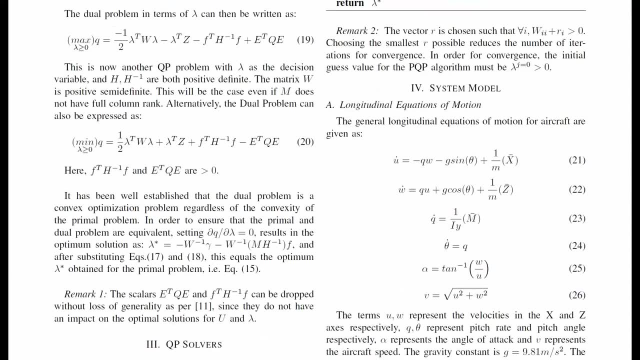 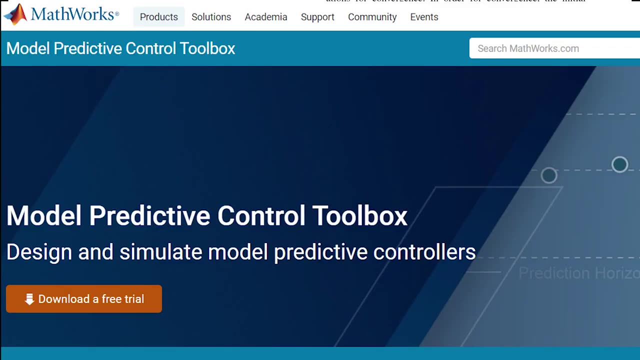 have those, you can proceed with the optimization. so then you have to use a solver now in MATLAB. you have. you have to use a solver now in MATLAB. you have many solvers which are built in. I believe if you have the MPC toolbox or any control system toolbox, they contain solvers for optimization. however, for now, 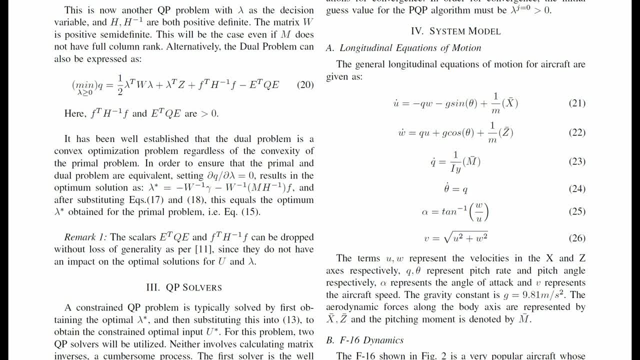 we'll be doing it from scratch because it's a good way to, and this is a linear method, it's not a nonlinear method. so for linear methods, it is quite simple to do it yourself. the solver which you'll be using is the parallel quadratic programming algorithm. this was designed at M E R L. it's called Mitsubishi. 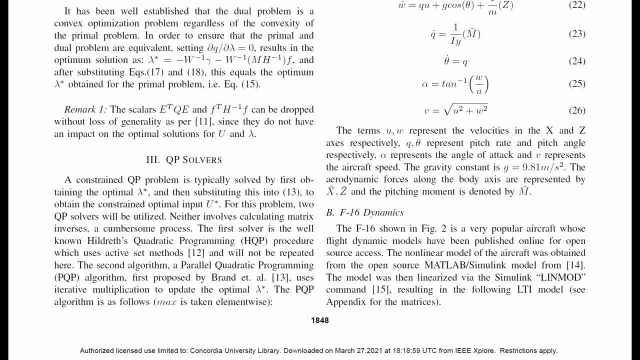 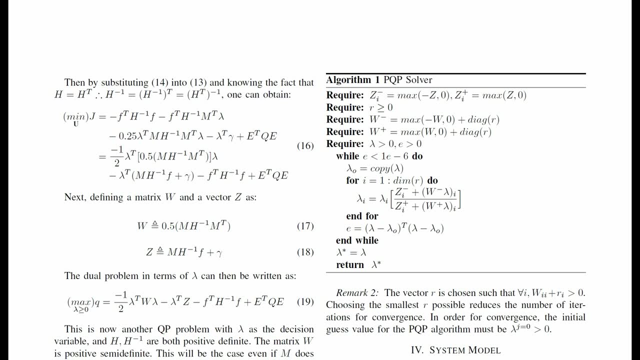 Electric Research Labs. this is a very nice research facility in the US and they do a lot of work in controls and optimization, machine learning, all those things. so this is the parallel quadratic programming algorithm here. I took it from the paper and I put it in this format so it looked nicer. and then you 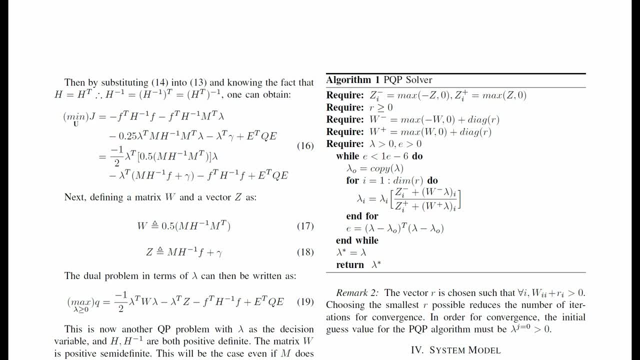 can see how it looks like here. so you have to. this max operator is taken element wise. I'll get into more of the solver when I show you the model, but for now i've just taken note of this algorithm. here you have to start off with w and z, along with some. 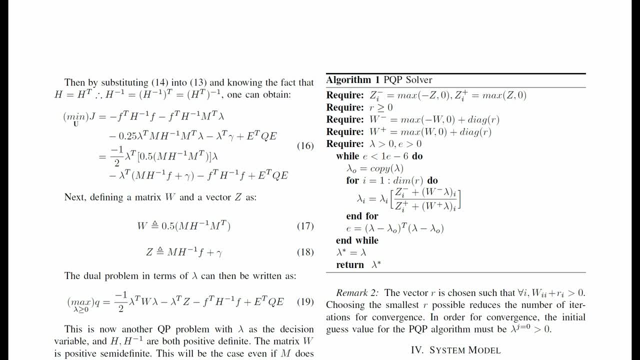 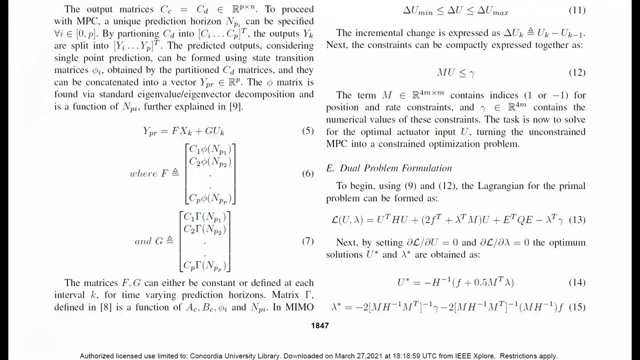 initial conditions. and then you have to go through this loop and solve for the optimal lagrange multiplier. so that'll be lambda star, and when you get lambda star you return that and from this lambda star you can then solve for u star. so you you take equation 14 and you put in this lambda. 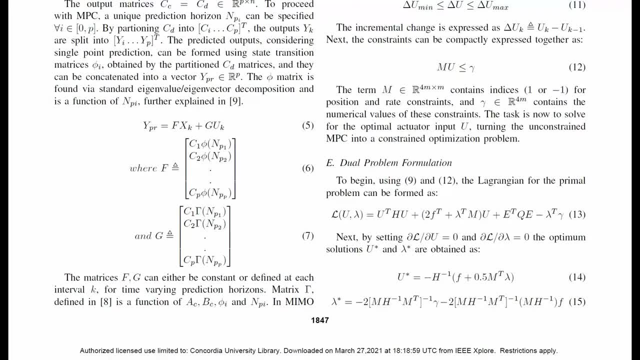 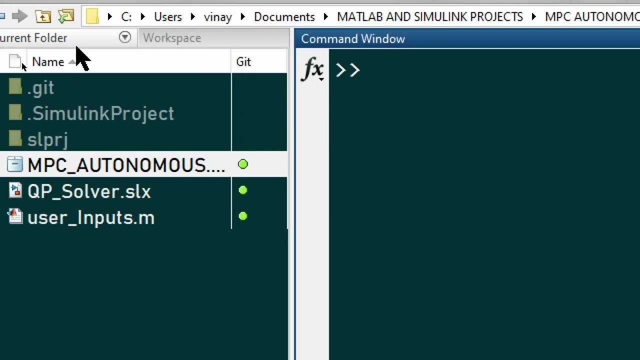 star there and that gives you the optimal inputs, and i will demonstrate that, and it'll make a lot more sense to you. so let's begin. so when you download the files from github, you will see them like this: first thing you want to do is you want to navigate to the folder. so in my case it is in: 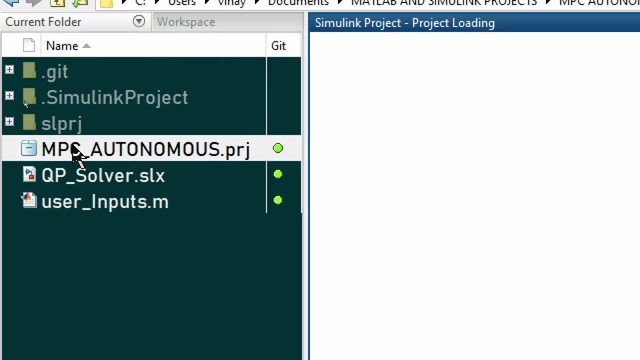 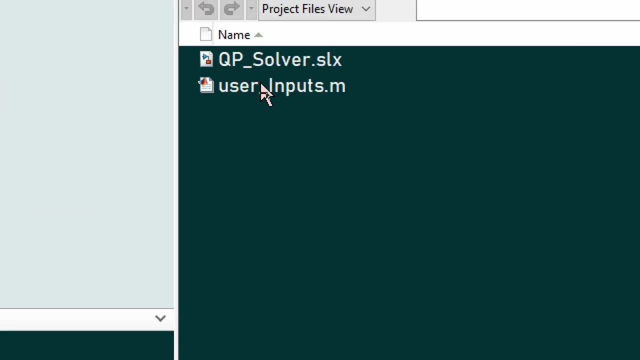 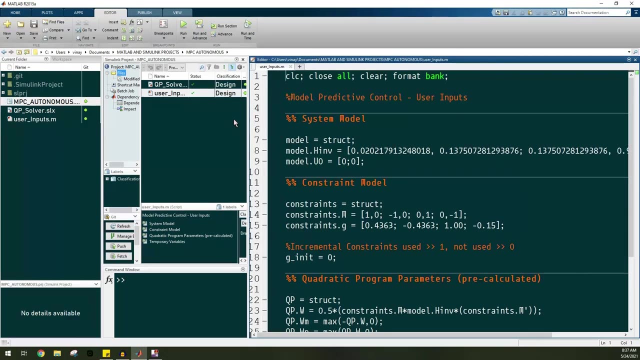 here and open the prj file, so that should load these two files here. the first thing you want to do is you want to load the inputs into the workspace, so open up user inputsm and you will see it there. so essentially i have some parameters already defined here. h inverse is from the paper. 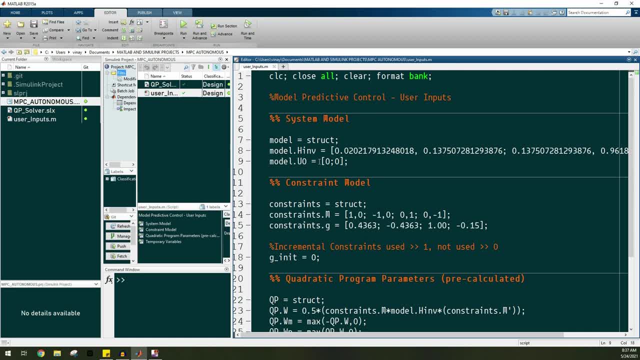 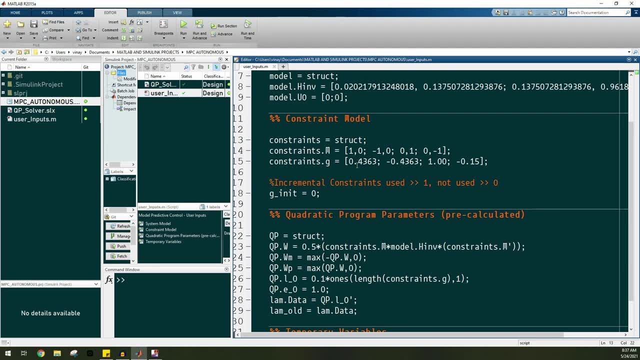 i just took a value here i have. so in this case i have a couple of inputs, two inputs. my constraints are that the first input is bounded between 0.4 and negative 0.4, and the second input is bounded between negative 0.15 and 1. so those are my constraints and m is 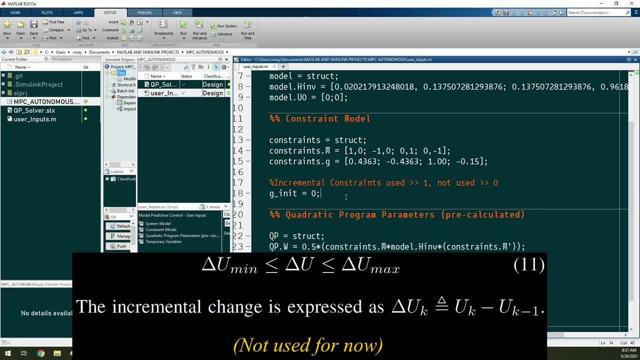 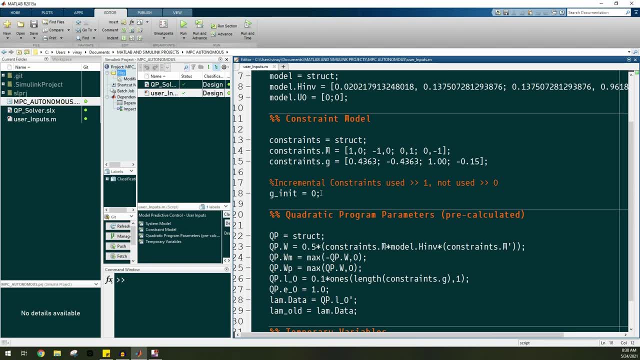 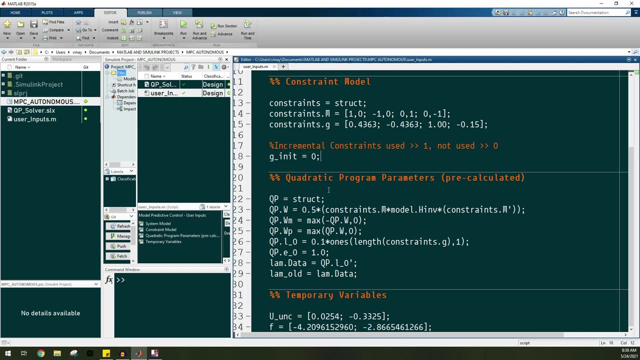 just a mapping matrix initially. i don't have any incremental constraints, so i just set this to zero um. i will get this. i will get more into this after. so, yeah, now i have my quadratic program parameters for the pqp algorithm. you know how i mentioned you need w and z, so in this case i have my w. it is a function of m, h, inverse and m. 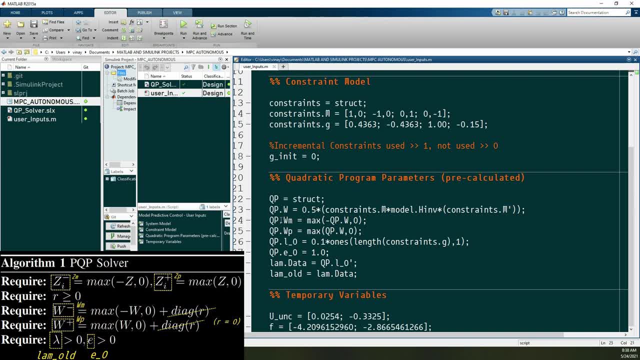 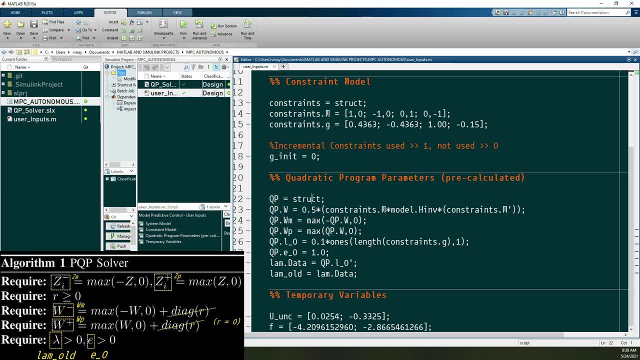 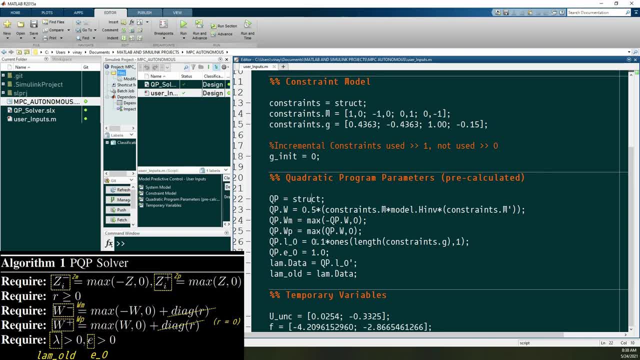 it has to be something which is more than zero. it's, it's 0.1, it's a vector of four, zero point one. my initial error should be more than zero because you want the error to be small, but it'll only activate the solver if the error is high. right, so you want it to be. 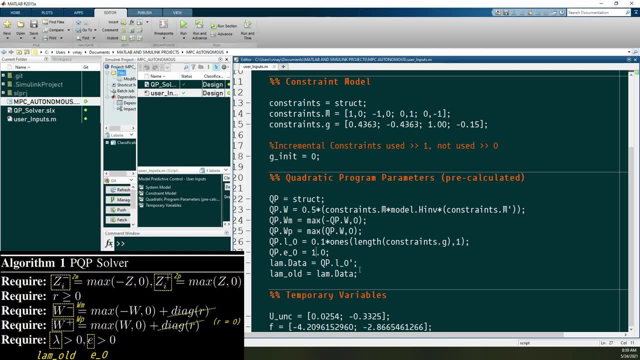 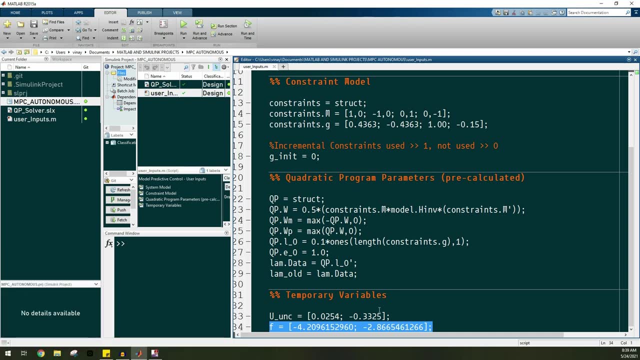 initially a high value and then it'll go down. and this is just a couple of more structs. i have to define the initial lagrange multiplier for now. my f variable is this: it is actually based on the control system error. i don't have my control system design now, it is just my optimizer. 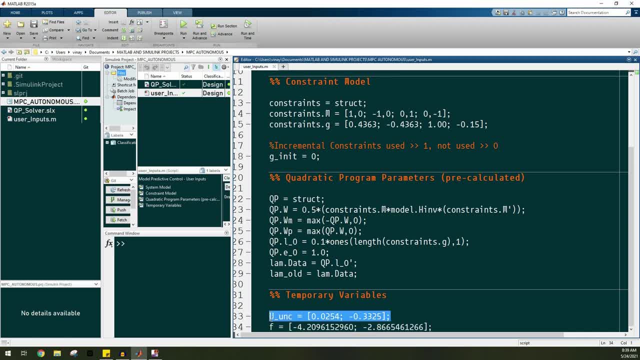 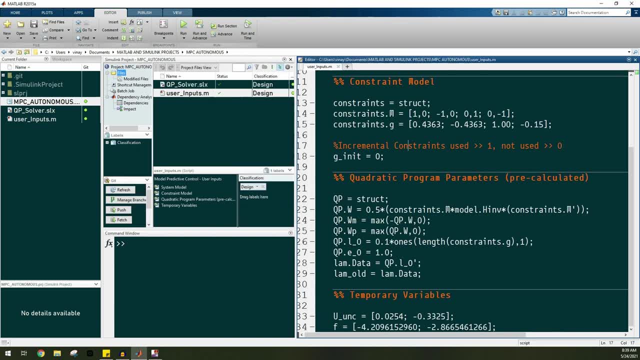 so i defined f there and i have my unconstrained inputs. so let's run this file first and let's see what we get in the workspace. so it's loaded in the workspace. you can see these trucks here. if i just type in qp, you can see how it's a struct it. 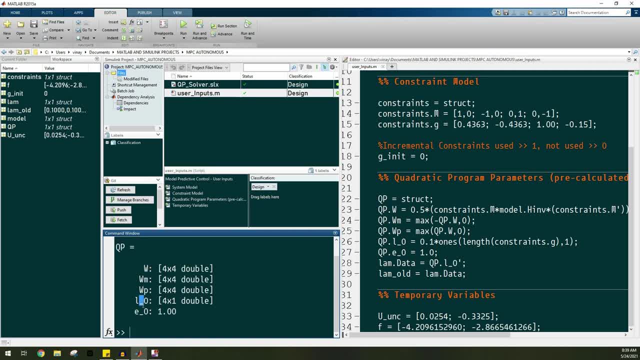 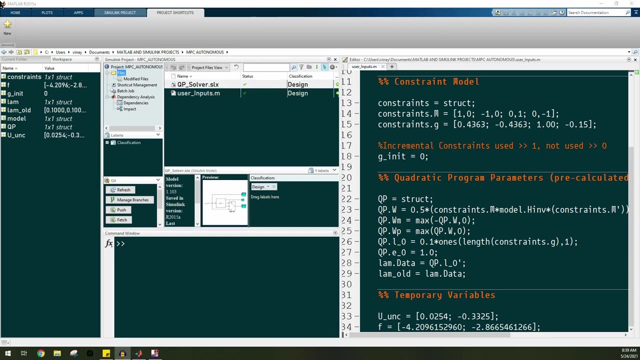 contains w, wm, wwp, the initial multiplier and the error, and then same with constraints. so it is a struct, all right. so, um, let's open the model now and let me explain that how that works. this is my simulink model. the first thing you want to do is press spacebar to make it fit the. 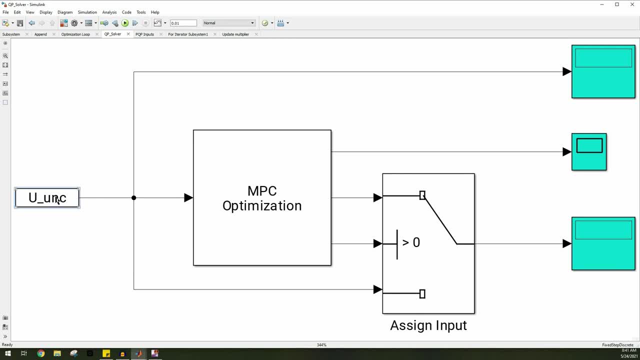 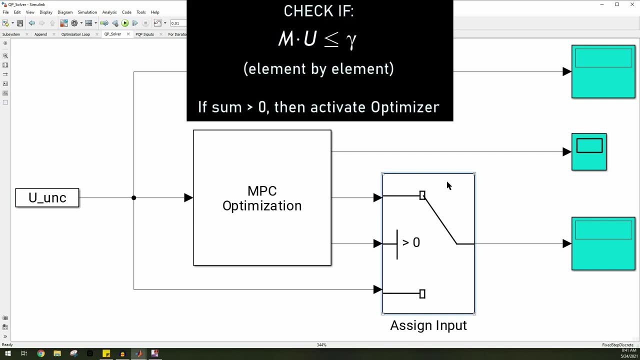 window. so this is my unconstrained inputs, and what this will do is this: will check that the inputs satisfy the constraints. if the unconstrained inputs meets the constraints, it'll not activate the optimization. it'll just pass through this here. however, if it does not meet the constraints, which which is in this example- it will activate my optimizer. 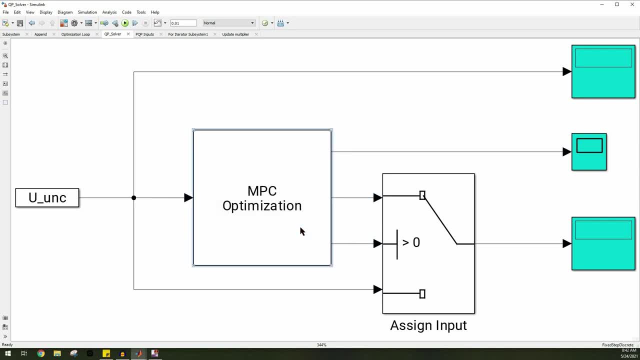 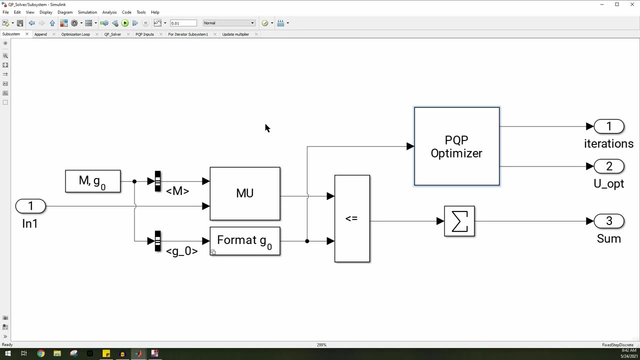 this is a subsystem. if you do ctrl m on this, you can see that into a mask, so that's why it looks like that. it looks a lot nicer this way. so if i open this one up, i can see my optimizer here. let's first look at the solver. 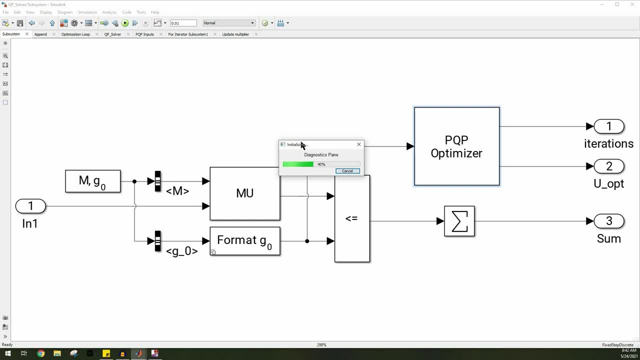 since i'm using a discrete time simulation, my solver will be discrete step of 0.01 seconds and i will only do one time step, so my ending time will be the time step, which is 0.01 seconds. right so? and that is because my model will be done in discrete time, not continuous time. 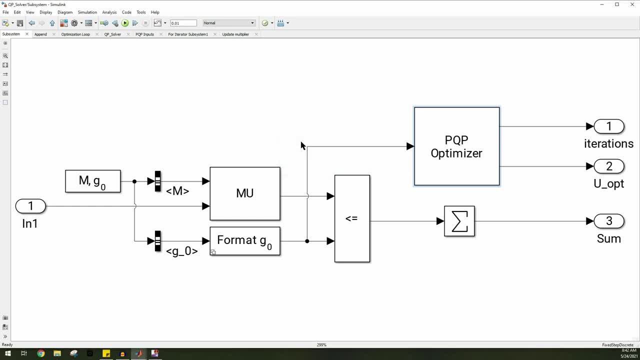 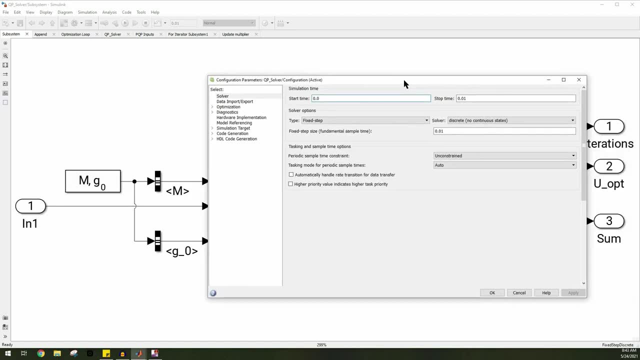 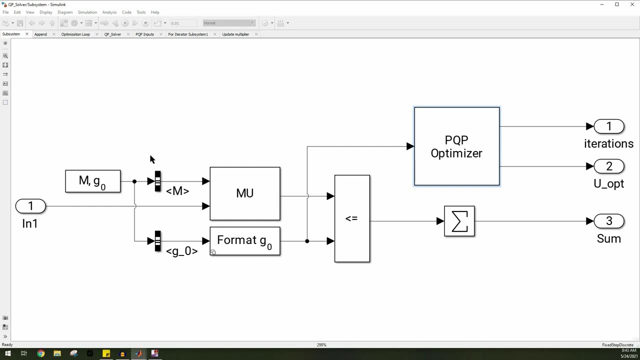 so all you have to do is make it very simple for the simulink solver to recognize that. so there you go: make sure it is fixed step, your step size is 0.01 seconds and it is discrete time and mapgov very simple and you don't have to worry that I'm 개�ญ. diamonds. 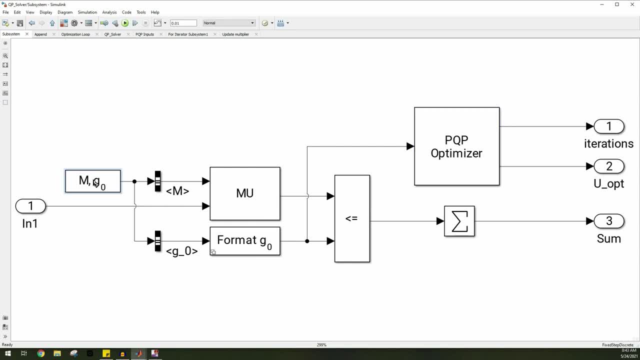 anymore to open with this design, so that gives us a еnormous přer состоîne. all right, so, with that being said, over here I have my optimizer, I have my constraints there. يLL, so that's γ from the paper you use a bus selector to select m. 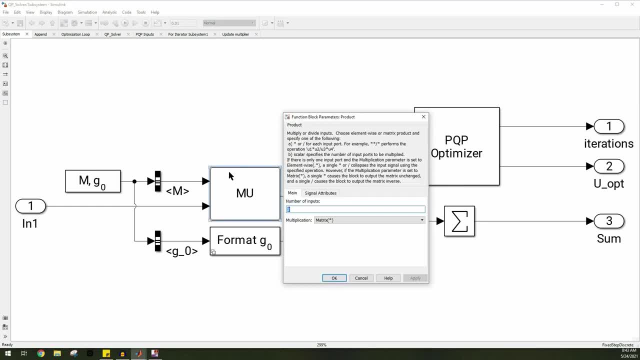 so if I open this one, you can see how it is a bus selector block, and then I just select Brother multiply m by u right, and then i use format g0. so this one here is a variant subsystem, because i may use incremental constraints or i may not, and in this case i don't, but i did it. 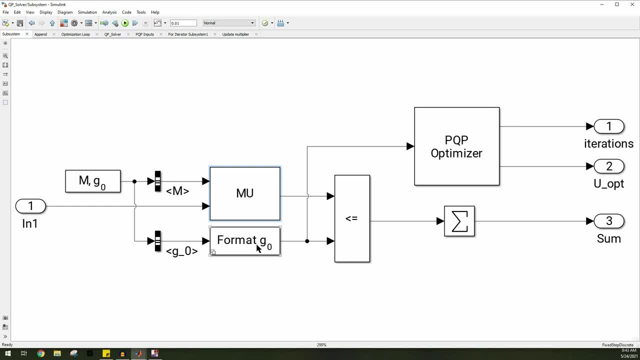 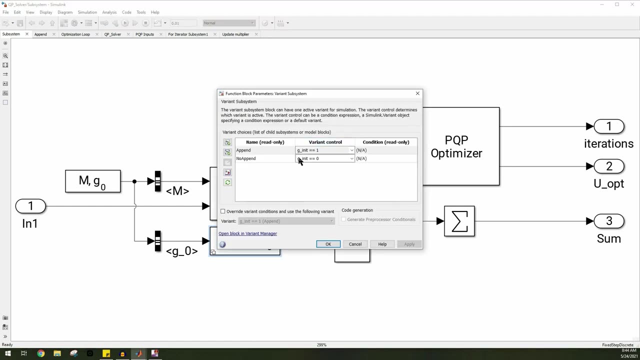 this way because if i do it after some time it'll just activate this one. so now i will explain how variant subsystems work. so right click on this and select block parameters. you can see how it's a variant subsystem. i have two inside append or no append. 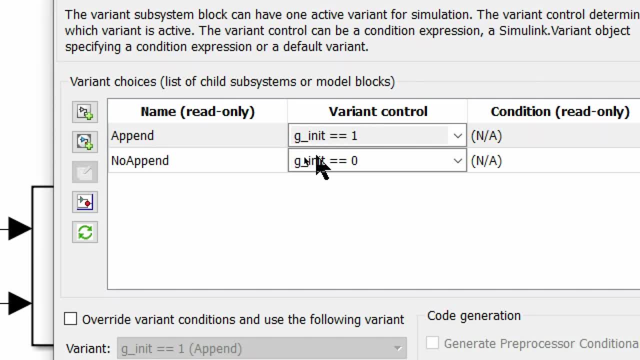 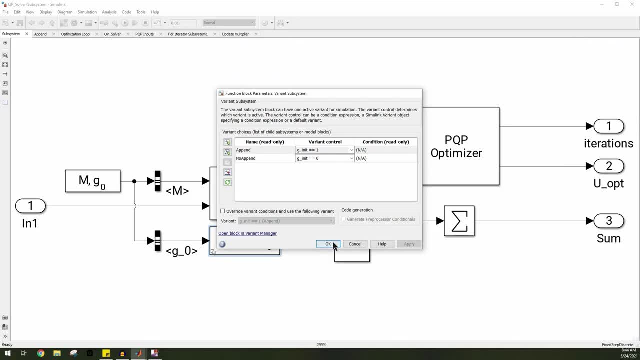 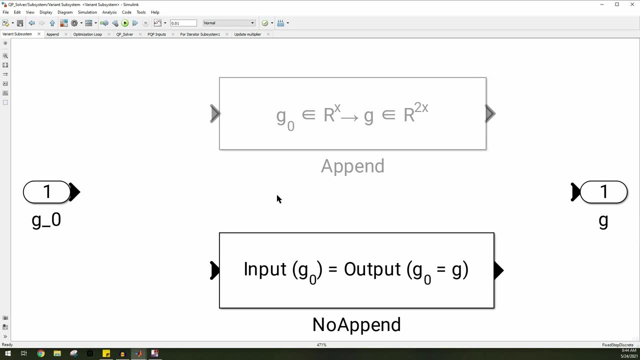 and this is my variant control, so it'll it'll activate either of these based on the value of g underscore in it, press ok and then let's open it now. so you can see how i have two inside here. i have g0 and g. you have to make sure that inside your subsystem here 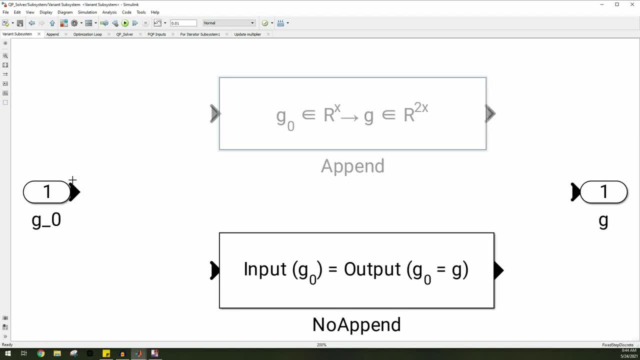 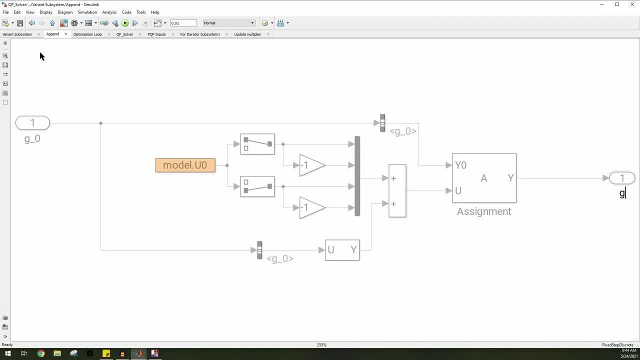 you have to make sure that inside your subsystem here you have g0 and g. you have to make sure that the inputs and the outputs have the same name. so here input is g- 0, output is g. in the first one the input is g- 0 and the output is g, and in the second one it's the same thing. 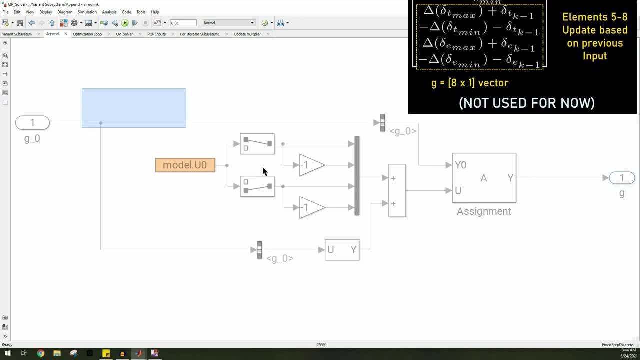 this one. what it'll do is it'll activate the model if i have incremental inputs, but now i don't, so it'll not activate this. but i can just explain this very quickly now. so what this will do is it'll do a u minus u at the time step beforehand, so it'll be uk minus uk minus one right. so this: 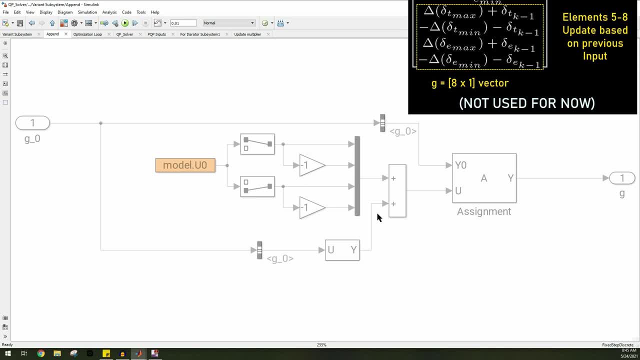 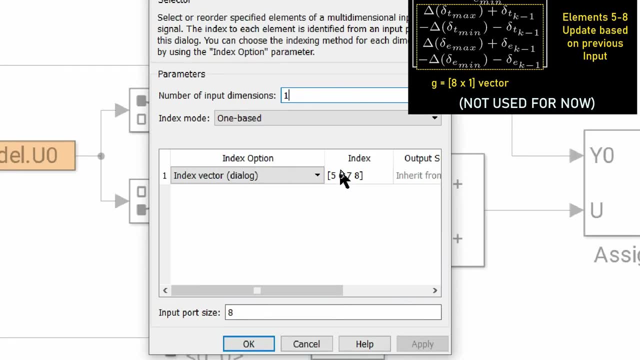 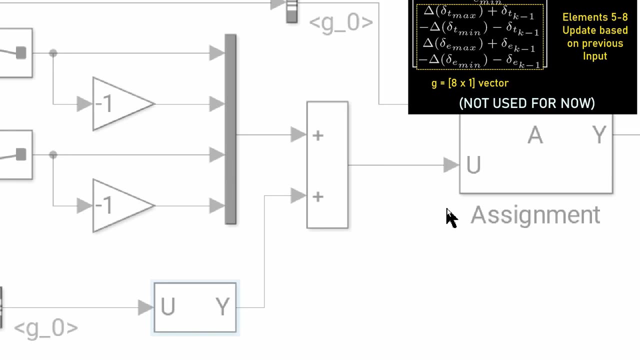 will select the top and the bottom, it'll just concatenate the array. so for this one i use the selector block to select the last four elements of g if it is an eight by one vector, so five to eight. it's a size, eight inputs in this specific example, my assignment block. i just assign it. 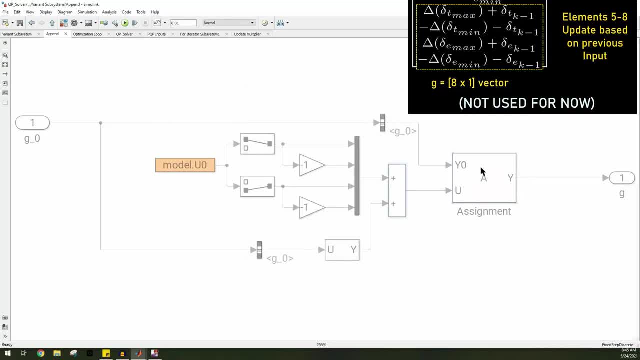 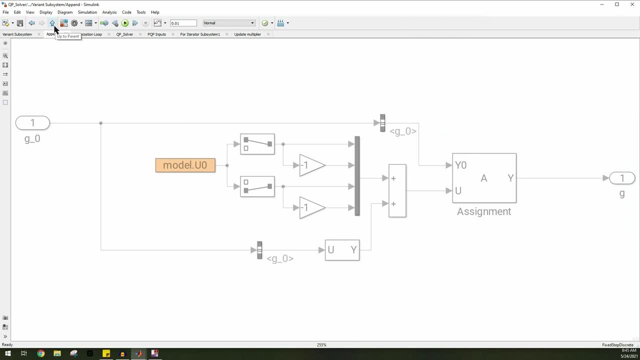 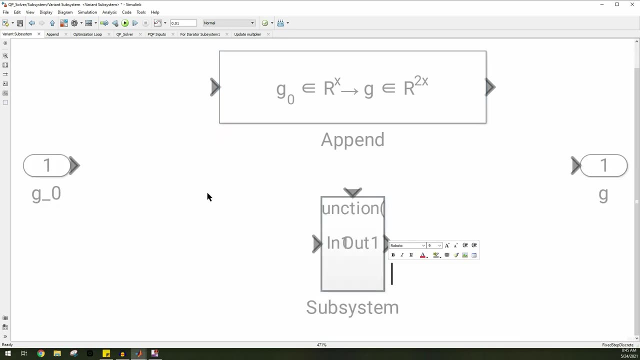 there, so i just add it and then assign it. if you see the picture which i put up, then you will understand better. but for this case i don't use it right, because it's just there in case i need it. so it'll just pass through this one here. so just sorry. so it'll just assign the output to the input. 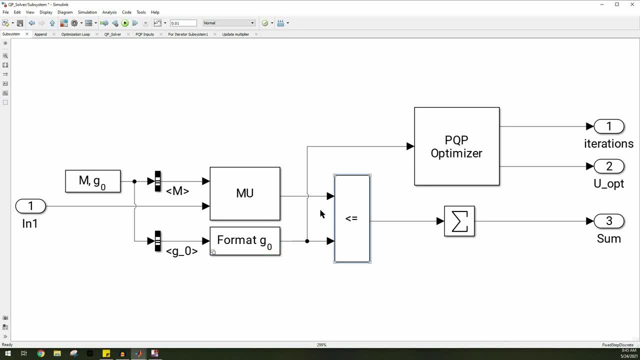 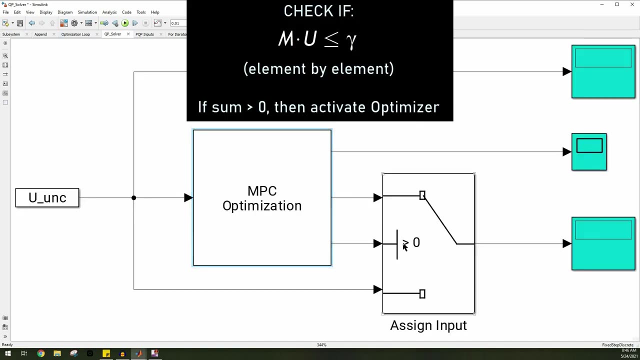 so that's what we use now. this will just compare m, u and g. so this compares the constraints and the sum value will just sum up all the values. now, if the sum value is more than zero, that means you do not satisfy the constraints and that is a boolean, so you just run it here. 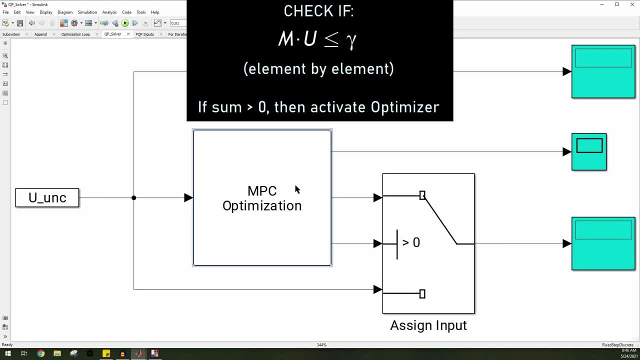 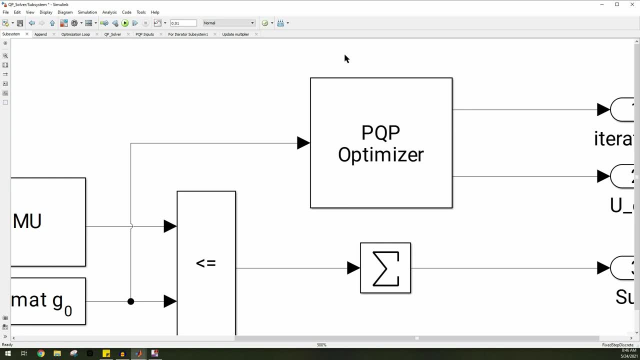 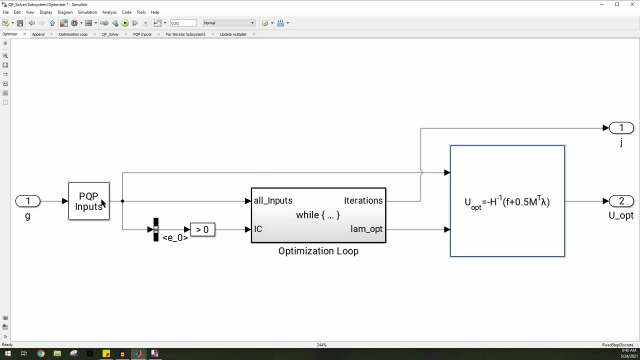 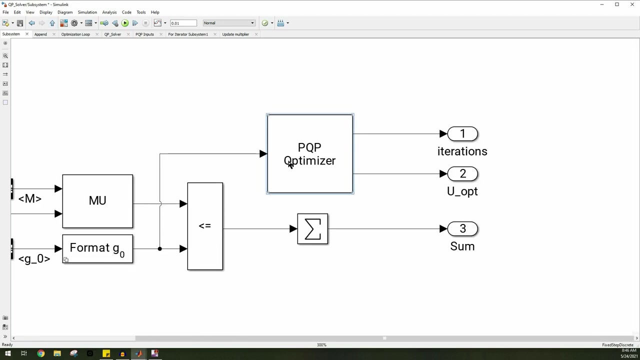 that's your condition, right? so you want this to be zero, to not activate my solver. this here is the optimization. so this is where all the magic is done. you can see if i open it i have- let's start off with the inputs. so i extract g and then put it into my optimizer. i have my inputs there, so that's all my. 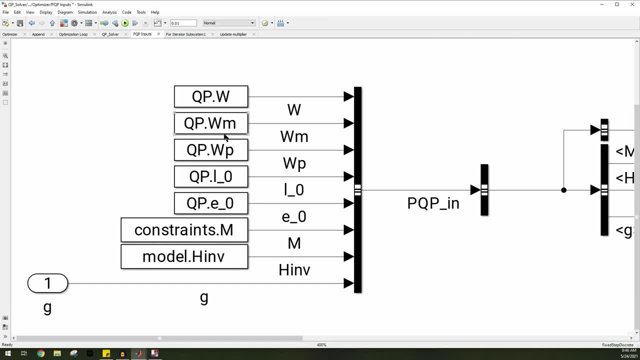 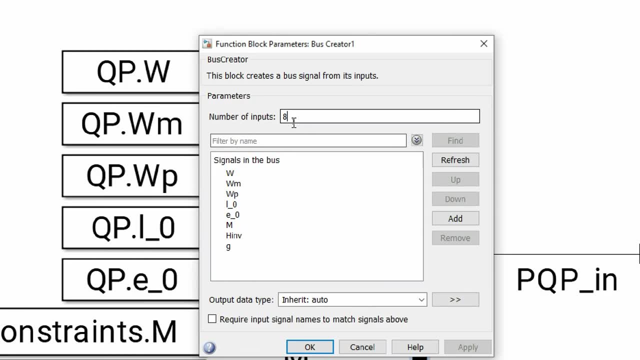 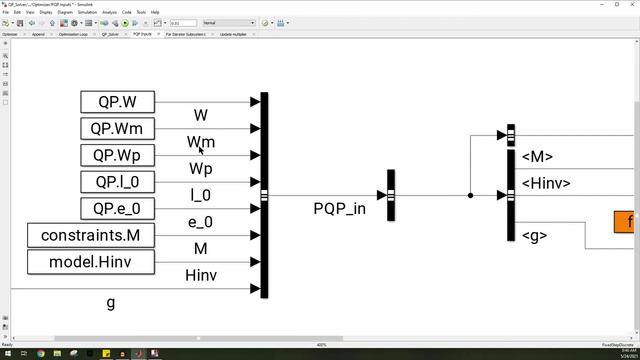 w and z's and all that. so w is here, wm, my initial multiplier. my error: i made a bus object. if i just click on this one, you can see how it is done. this way i have my signal names. i make it into a bus called pqp. underscore. 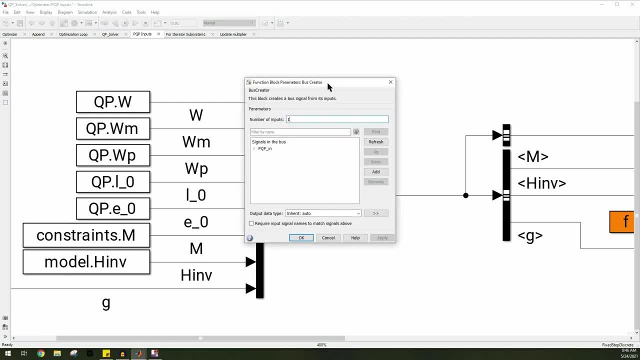 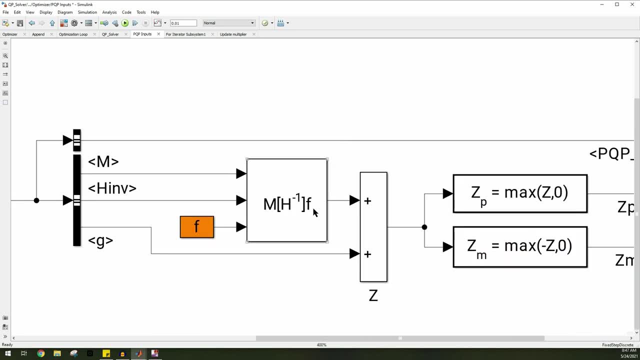 in that this one is also a bus creator, and then i just select i first, i do m, times h, inverse, times f. f is from the workspace, so i just use a constant to pull the value inside. i just select m, h, inverse and g there. so i just select it this way. 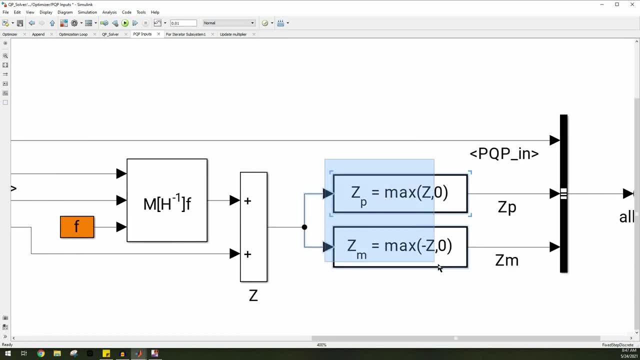 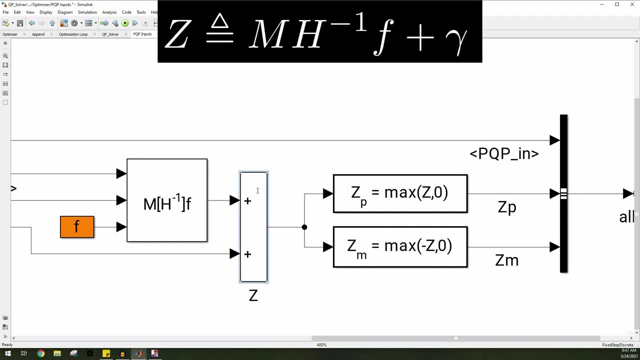 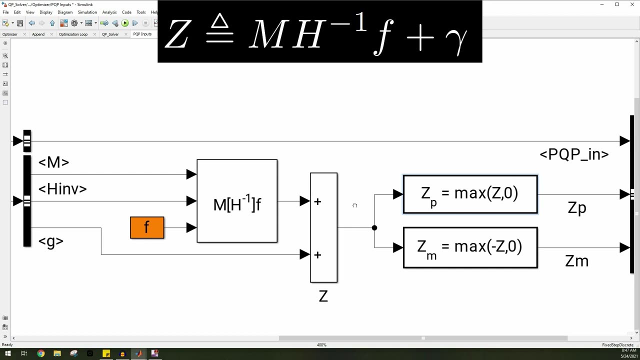 once that's done, i actually form up z in here. i solve for z, zp and zm because we need this in the optimizer. so z is over here, right, so it is m, h, inverse times, f plus g. if you see, in the paper i form up zp, so this is basically a max operator. so for this one, 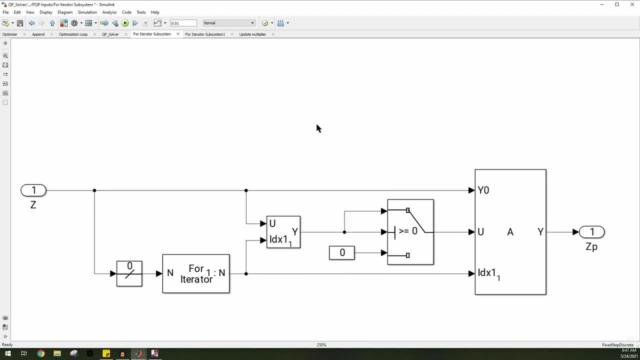 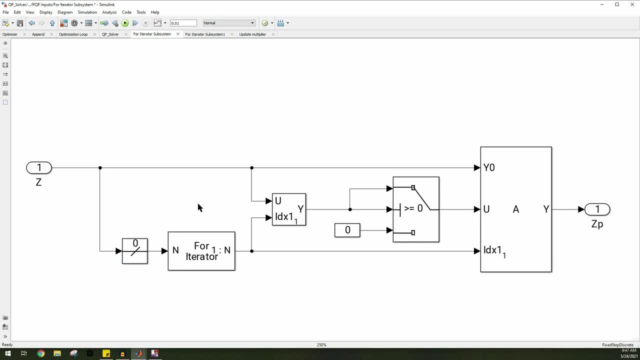 if you, this is a subsystem, so if i click on this one and if i open it, so this will take the width of z and that is how many for loops you have to do, because in this case z is a four by one vector, so you will have n equals four. and then you have a four by one vector, so you will have n equals four. 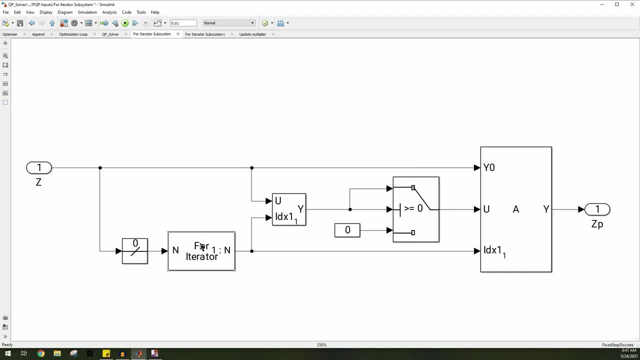 when i compile the system, you will see this value change, and for this one i select each value of z and i check it. so here it's: selector. i'm selecting each value of z. it is a four vector, so i just put four in there and then i compare it to zero. right, this is a switch operator. i'm comparing it. 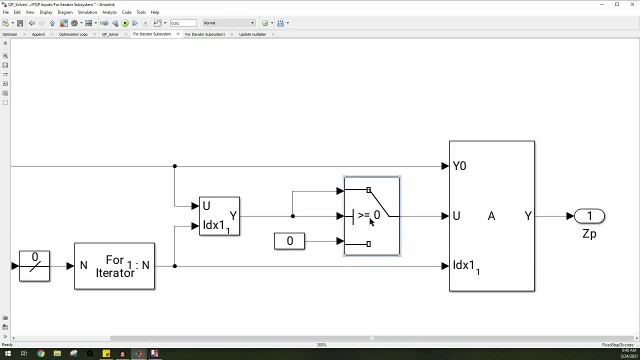 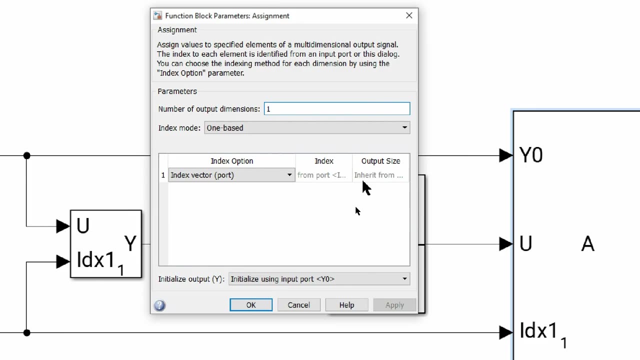 so if it is more than or equal to zero, then it'll pass through input one. otherwise it'll pass through zero here. so i'll just reassign values of z. this is my assignment block. so for this one, i just all you do is you put this into a port index: vector: port: select this option here. output. 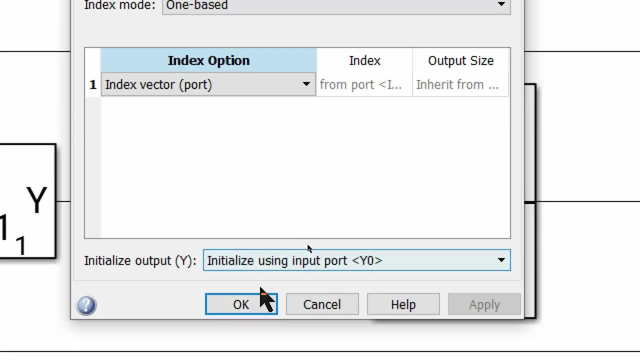 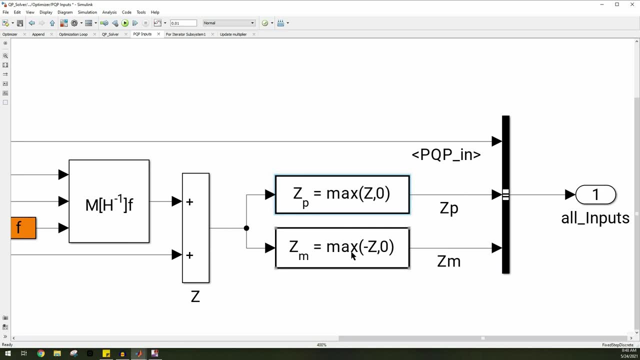 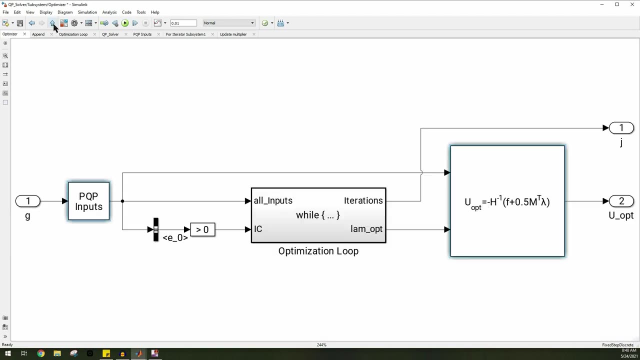 dimensions, one that's good- and then initialize it this way. so you just assign the values of z here back and you will get zp, and for zm you just put a negative one there. so you solve for w and z and then you put it into the optimization loop. 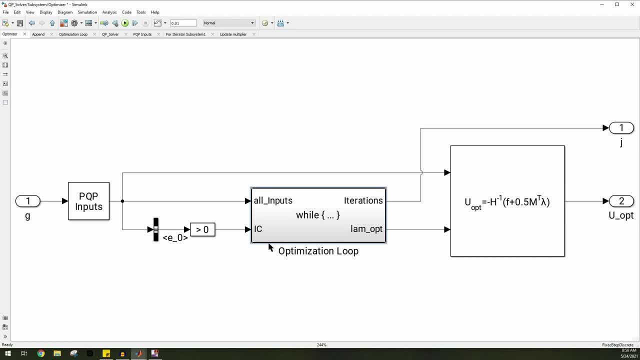 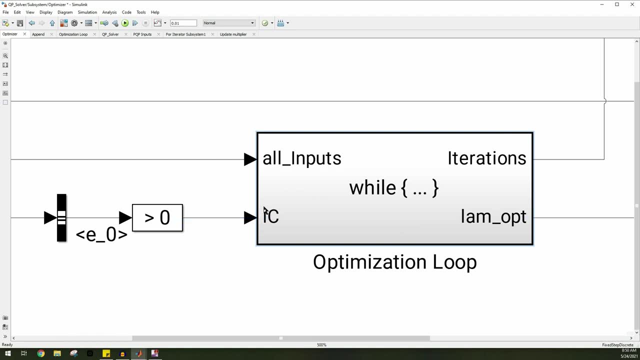 inside my loop, i select the error. so this is a while loop and a for loop is inside the while loop. so i make sure that my initial condition is that the error is more than zero, which it is, it will only activate when this is equal to a boolean one. so if i enter the subsystem, 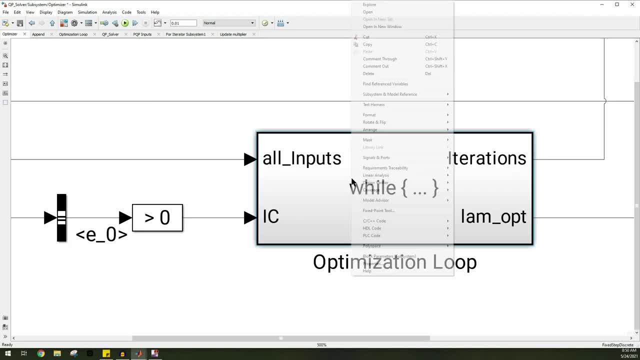 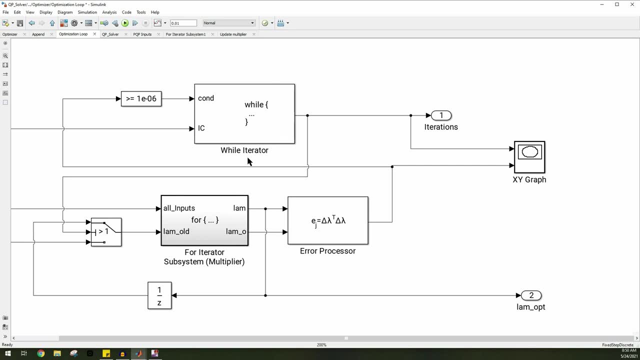 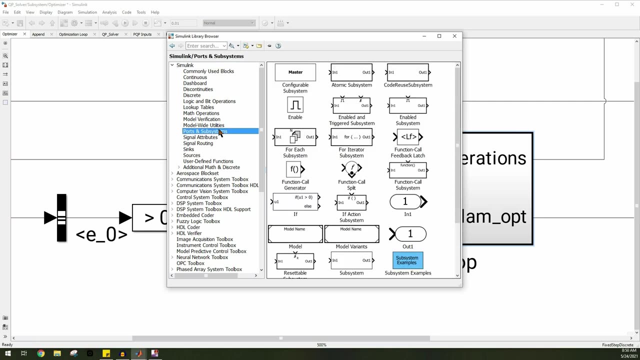 here. but if i actually first go back and if i right click on this one and if i select subsystem, it is just a normal subsystem and inside here i have a while iterator. so you have to drag in a while iterator browser if you can see here, just drag in a while here. so which is this one here? 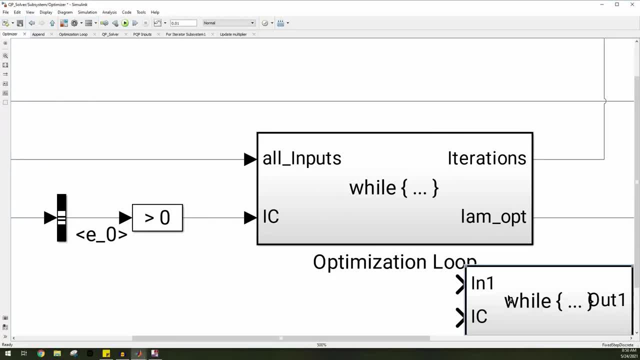 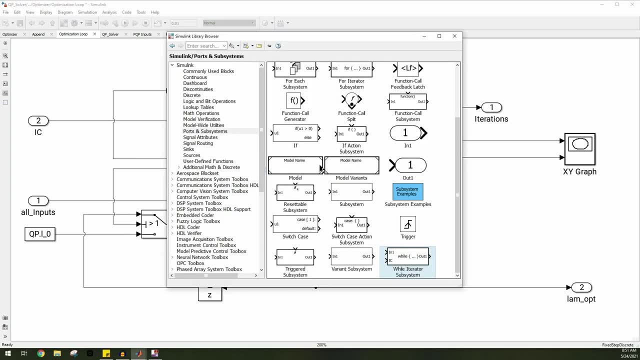 you just drag and drop it inside and then do all the connections there and inside this while loop. i make sure that i have a for inside here. so for this one it is again in the library browser. it is the for iterator subsystem. so that's this one here. 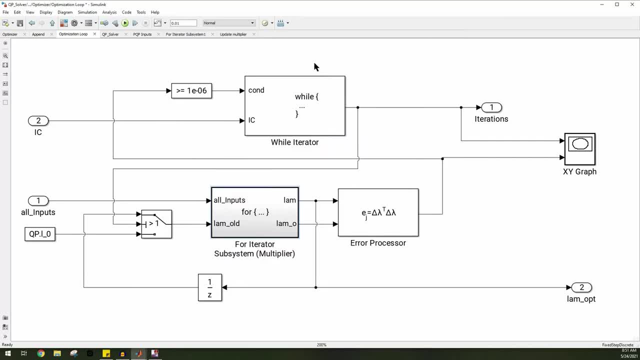 you just drag and drop it, but first let's explain this while thing. so the condition is that you want the error to be less than zero and or some value close to zero, which is 0.1 times 10 to the power of negative 5.. so it'll stop there. so, while this condition is not false, it'll just keep on going. 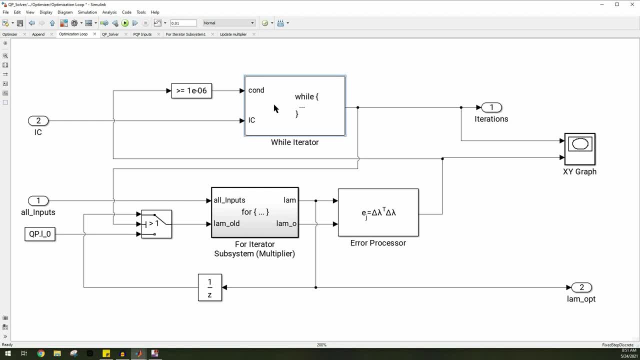 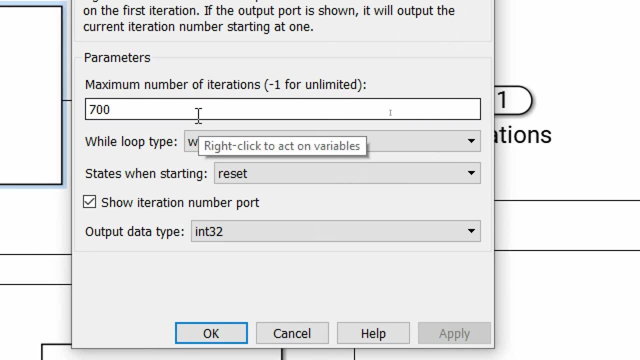 and the moment you you do not meet this condition, it'll stop the loop. so inside here i do have a maximum number of iterations, so this could be in the negative one, but then you may have an infinite loop, but you don't want that. so in most cases you have to have 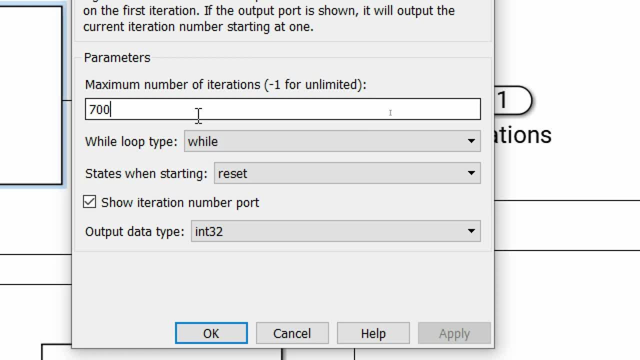 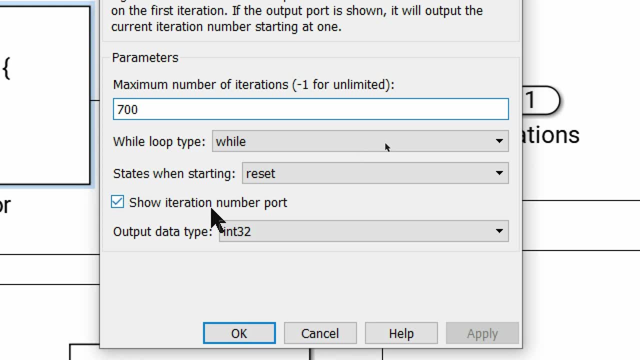 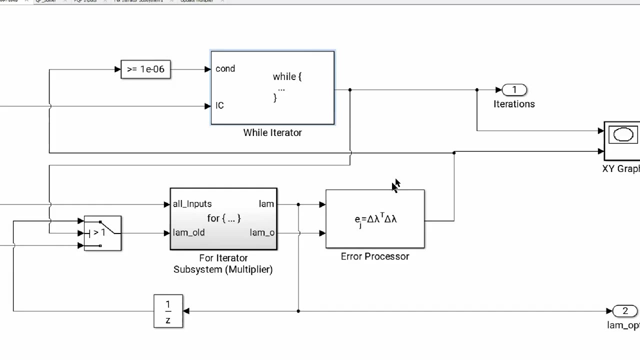 the optimizer converge. you don't want it to fail, so i just put 700 for now. i do have my. i do do this, so make sure you click that to select the iteration number port and i will show you why after and leave everything else as is. so that's my parameters for that. 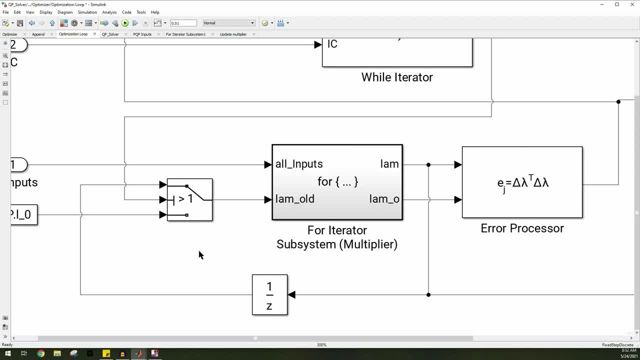 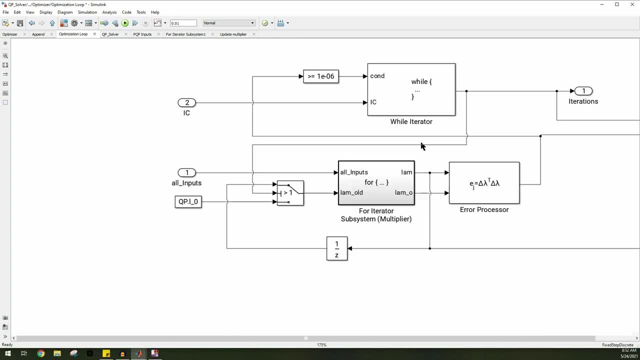 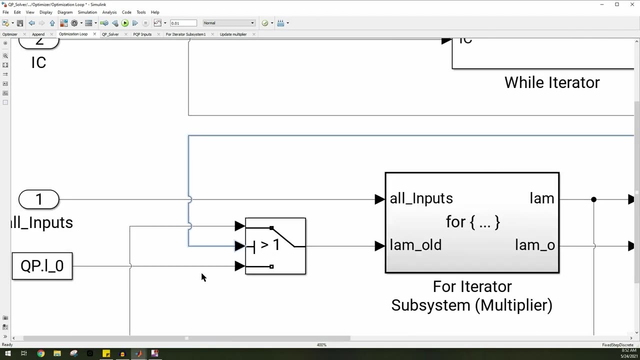 now this is where my loop is done. so initially at the first iteration, i have my initial lagrange multiplier. so you have to pass in this one here. so the iterations come out of this and they go into this comparison. so only for the first iteration you have to pass in this. 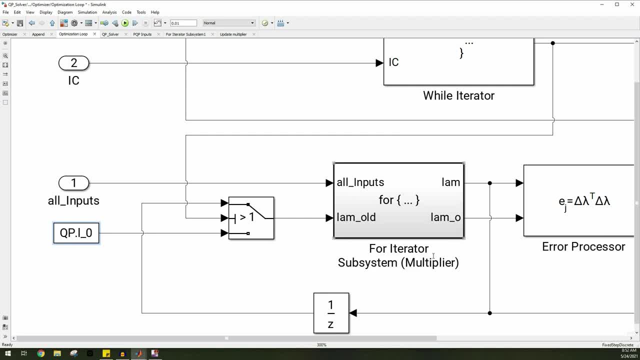 lambda, but then after that you will have to do all the rest of it will have to, you will. you will have to use the loop. so when iterations becomes more than one, it'll pass in the top input which comes out of my for loop. so now let's go into for block and 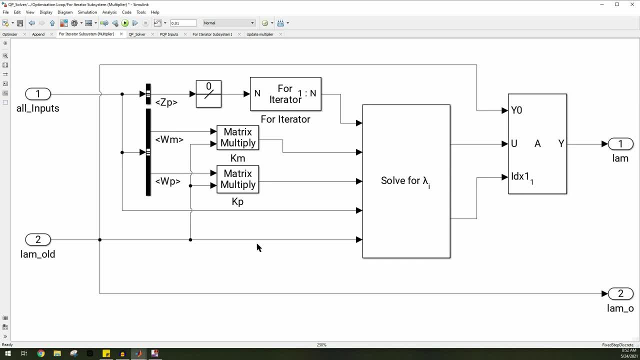 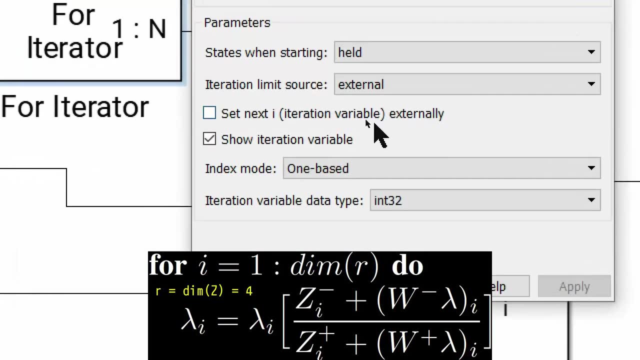 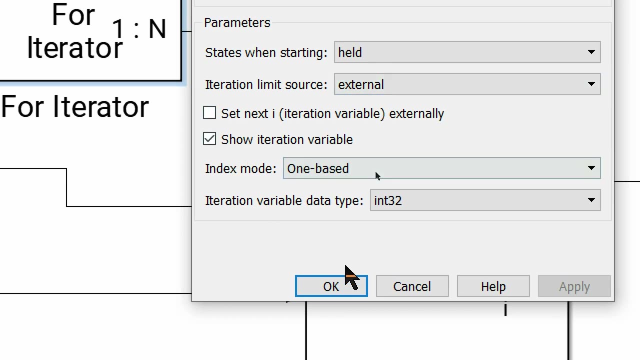 let's explain this one. so in here i do my for loop. so in this case i have a similar structure. i have my for block in here for this one. make sure your iteration limit source is external, because you have to pass in the dimensions from there and then you click show iteration variable there. so 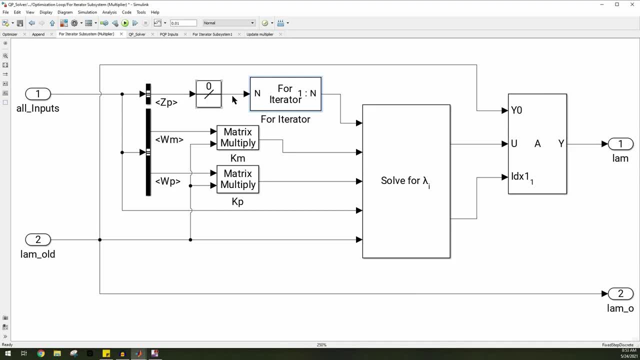 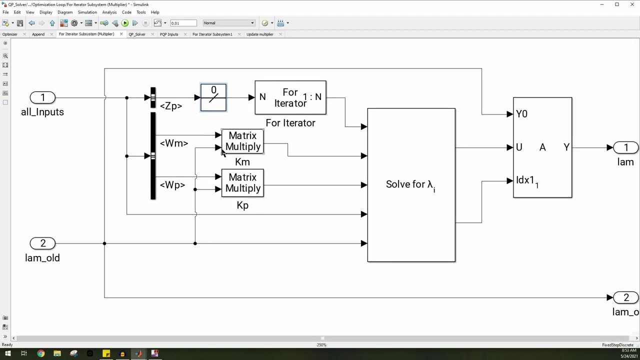 what this will do is it'll take in the dimension of z and that'll be your iterations maximum, so this will be four for this case. you solve for wm and wp based on your optimizer how the structure works. so you get all these parameters and then you solve for. 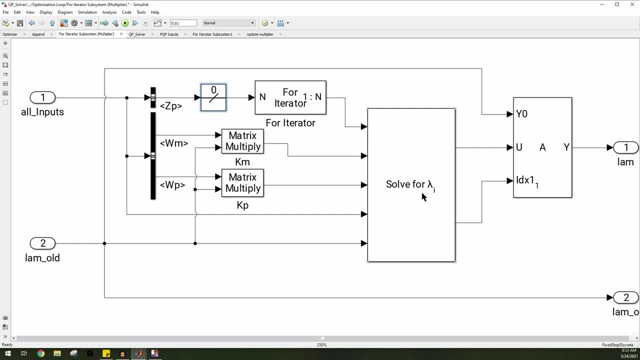 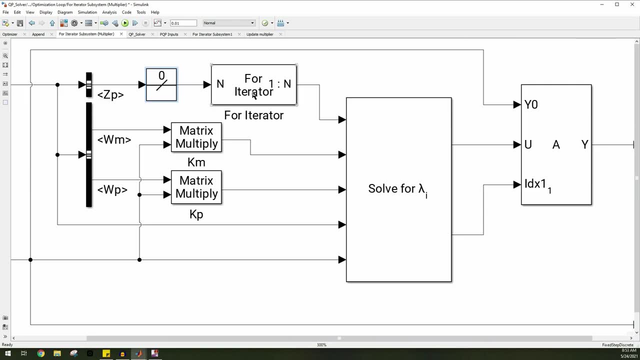 your lagrange multiplier, you have to update your lambda, but. but you have to update lambda, each element of it, so that that is why this index here i is from 1 to n right. so, yeah, let's go into this one and let's see how that works. 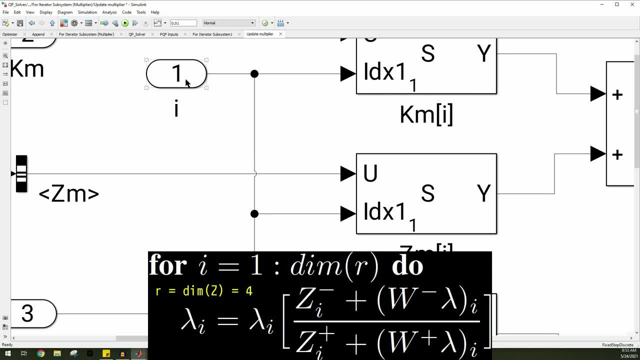 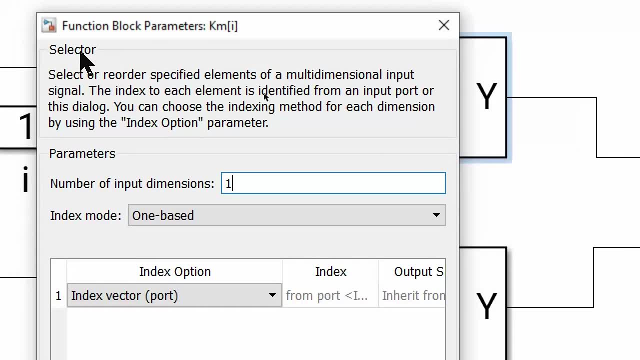 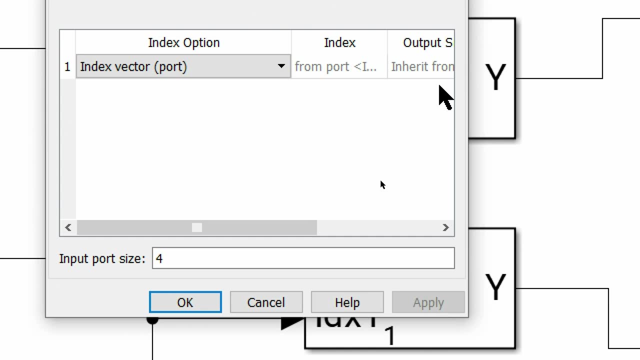 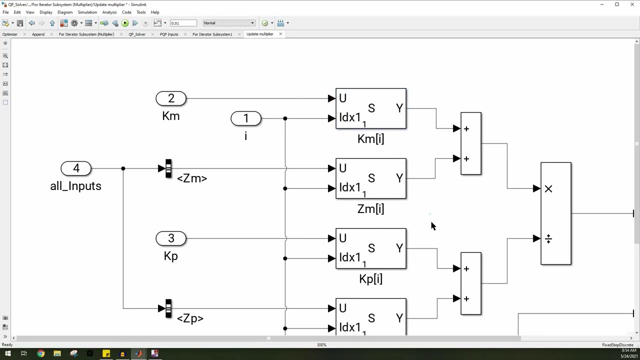 so i pass in my i, so i equals 1, 2, 3, 4 and you pass it in the index here. so so make sure the index vector is port, because you have to pass it from the outside or don't select dialog. make sure it's port. the input port size will be four because you have a four element vector here. 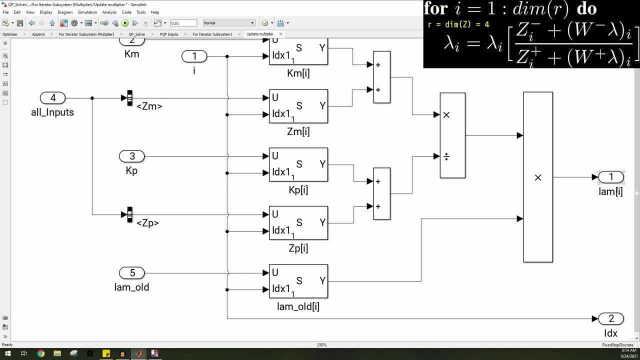 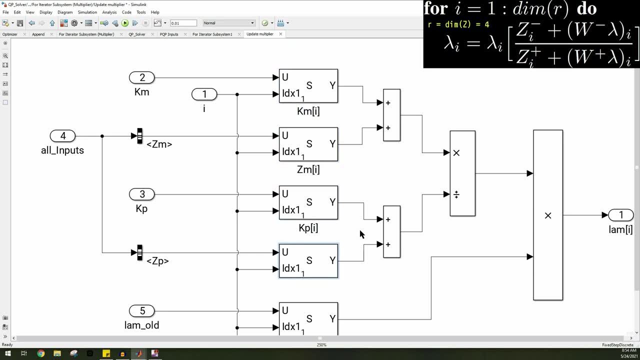 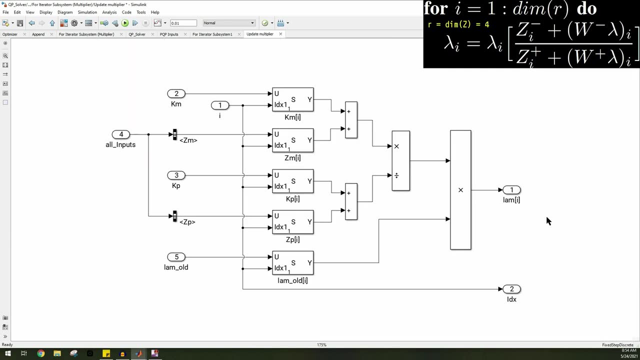 and when that's done, you have to simply calculate lambda i in this case. so you just pass an i all the way down and you use km, zm, kp, zp and then lambda old. so, based on the formula, you can see it's quite straightforward. you just update lambda i. the most important thing to know is that you have. 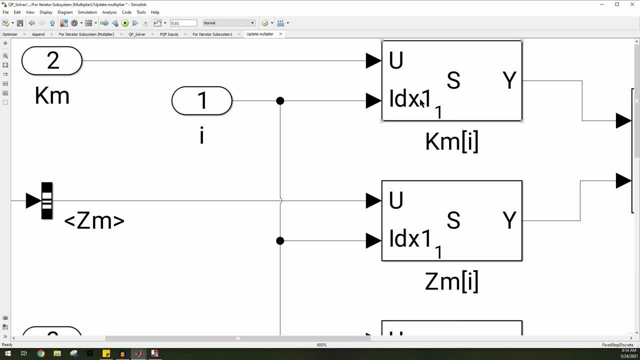 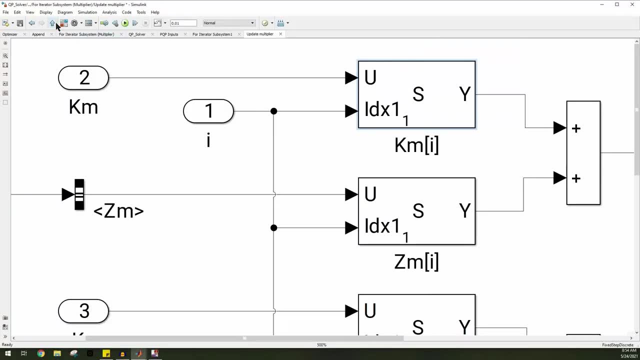 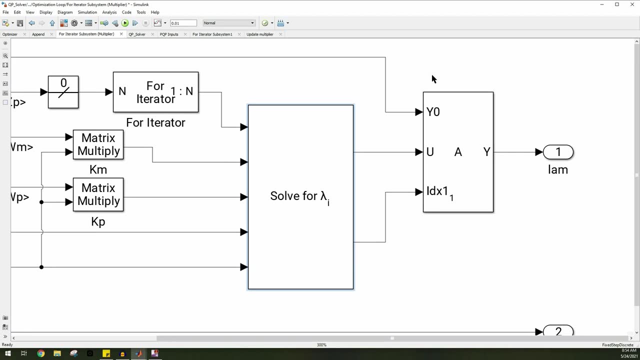 to pass in the iteration from i equals one to four outside. so that is why i mentioned to select this as a port, because it has to be passed in. so don't forget that. and then when you have lambda i, you have to update lambda, right, so that that is done via this assignment block here. so in this case, 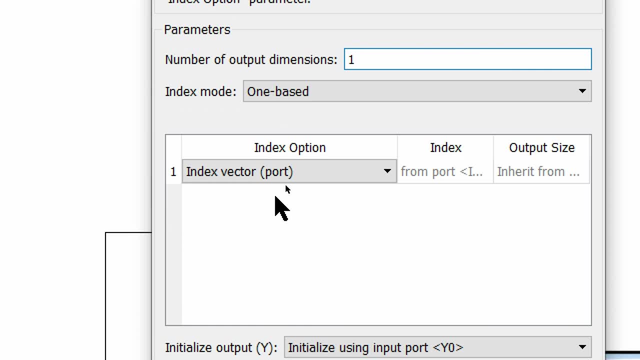 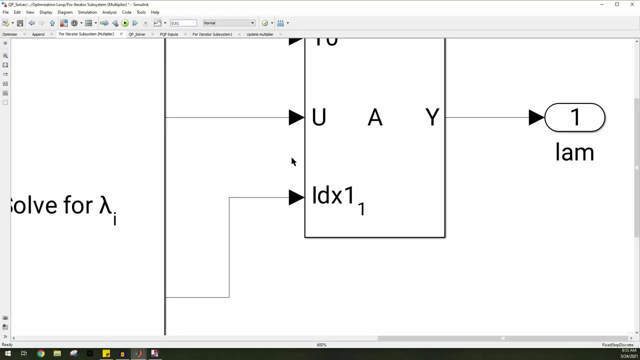 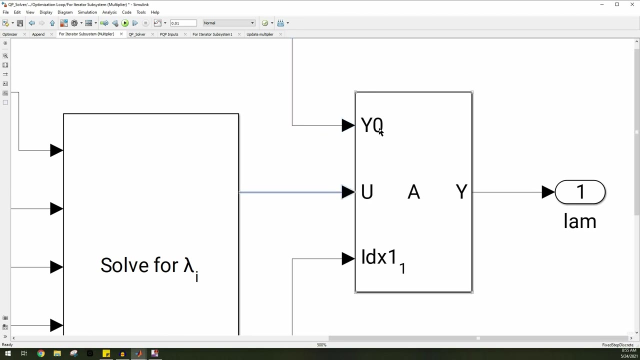 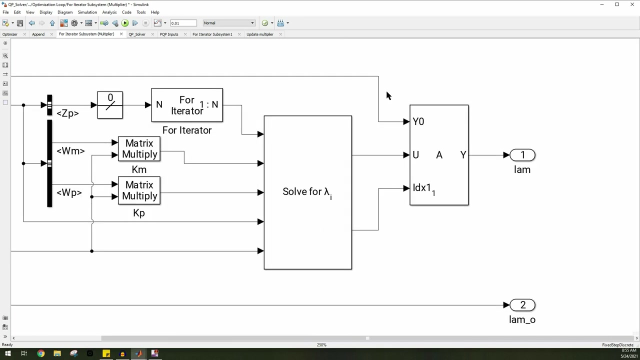 here i have. once again, it is a port. make sure it is all ports, okay. so yeah, i have my initialized output with this one. so what this would do is that that is my original output, that is my input, so it'll assign u to y zero. okay, so that is why my updated lambda goes into u. that's your update and that is your. 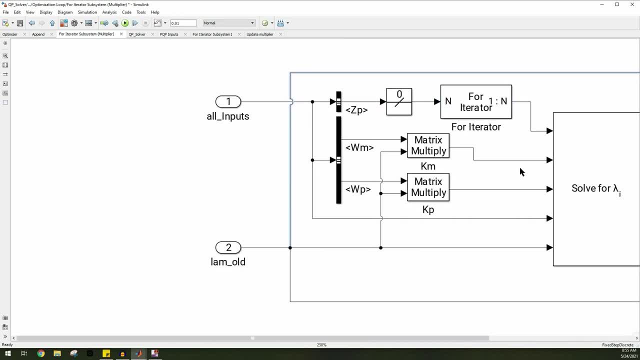 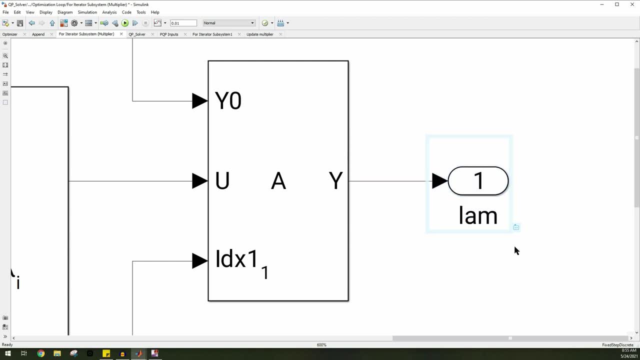 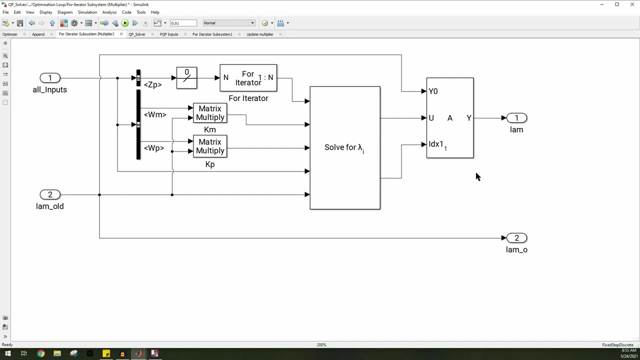 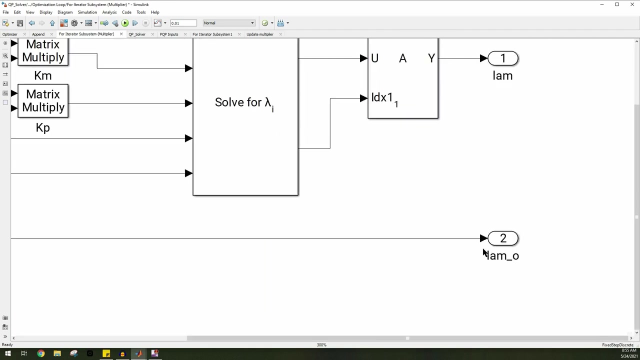 old value. you can see how the old value is simply lambda. all it's being passed into y zero, and then you will get why, right? so i hope you understood this very well, you that? so i have my, so i have my, so i have my in here. 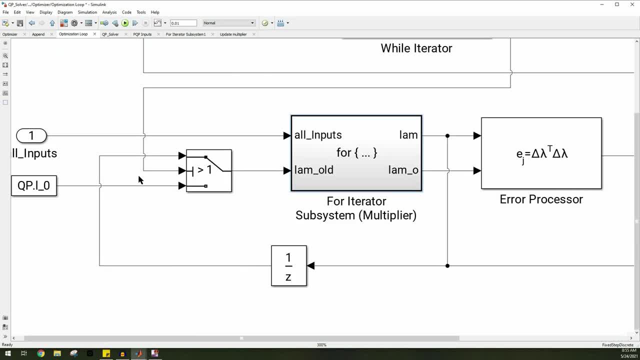 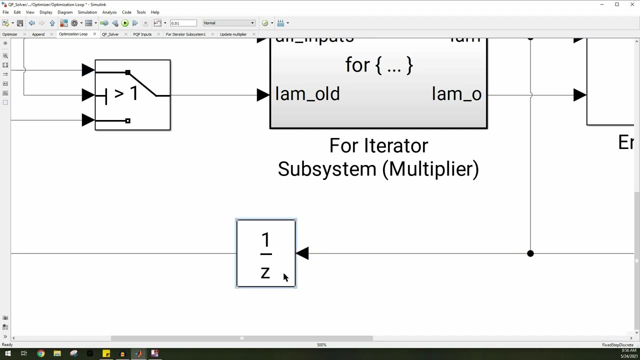 i also output my old, so i want to solve for the error. so i pass in lambda back inside because i need. so i pass in lambda back inside because i needed to update that at each iteration. so i have to pass it in this way, here and now. pay very close attention because this here is the deal breaker. i spent like six, like. 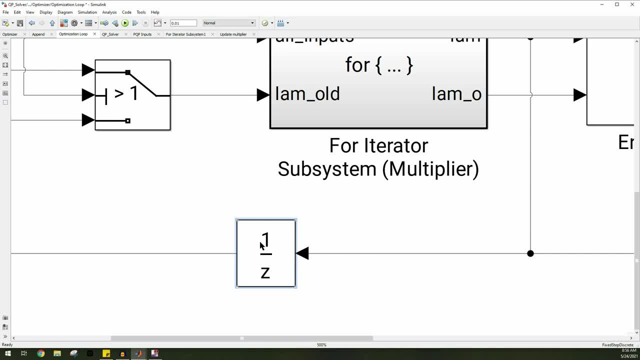 hours trying to figure this out and i was missing this unit delay block. if you don't have this, you will cause a lot of issues. so make sure you have it please, especially when you update the same variable again, because i spent like all this time trying to understand why my thing wasn't working. 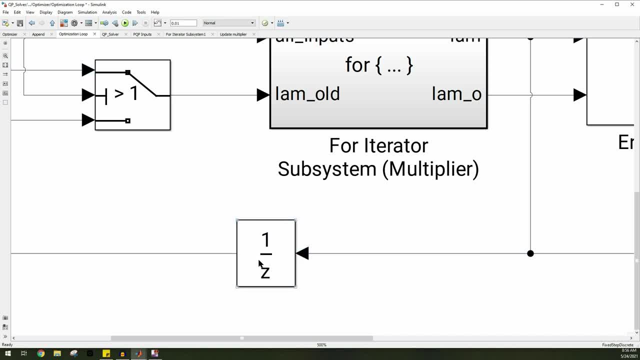 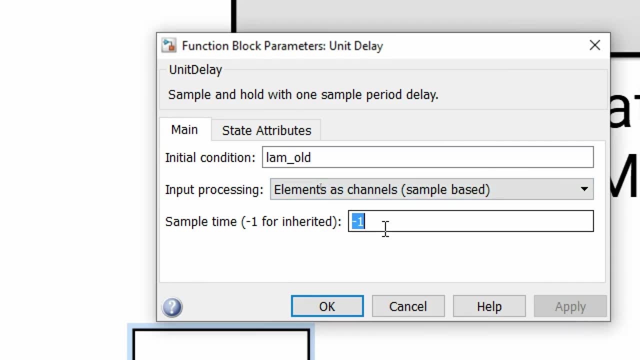 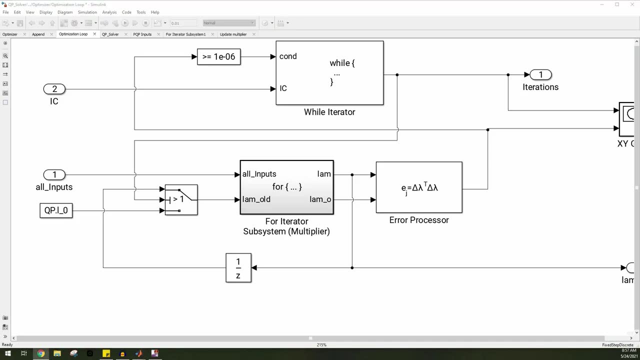 but i finally got it to work like after i put this one over z in. so this unit delay block make sure that the initial condition is lambda old and then the sample time is in the negative one okay. so that's very crucial. if you look at the symbol link documentation for unit delay blocks, you will 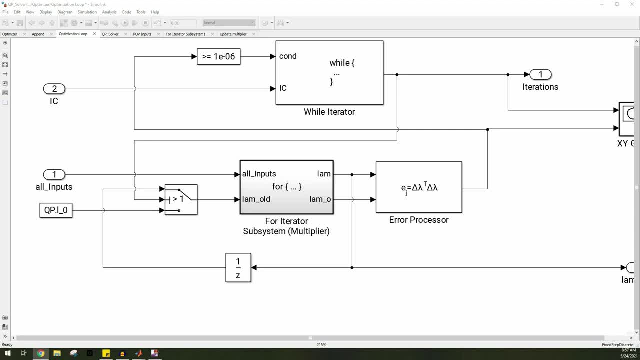 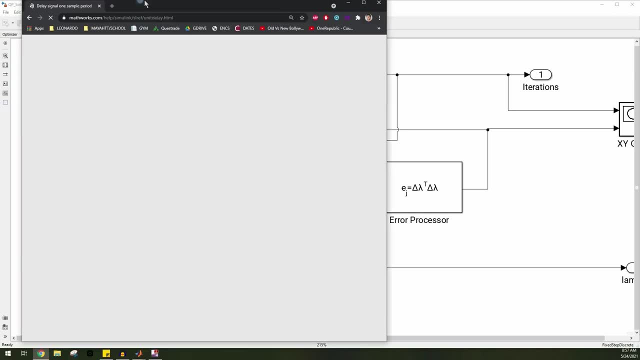 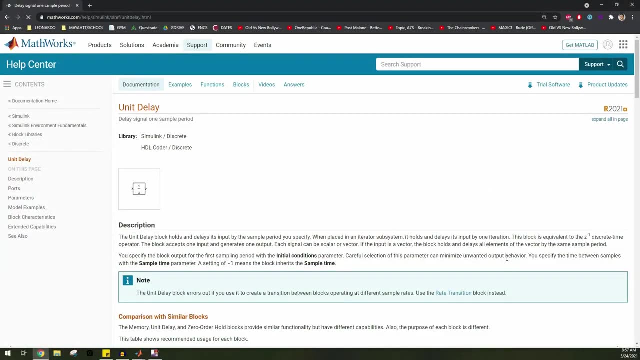 understand what i mean. so i'm just gonna quickly open that here and then i will show you. so look, so if you read this carefully, you will see what i'm trying to explain to you. so there, there we go. if it is an iterated subsystem, it'll hold and delay the input by one iteration. so so this is. 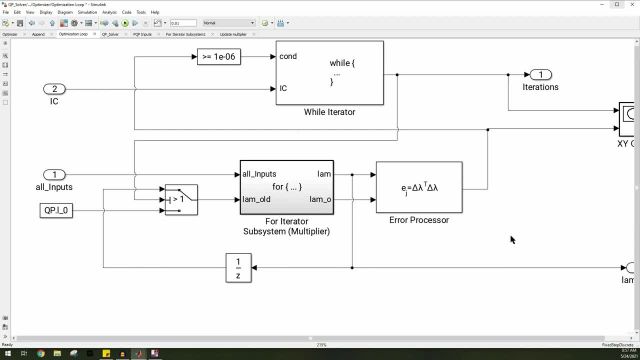 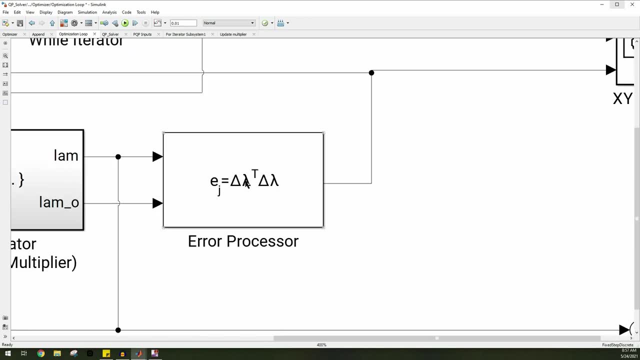 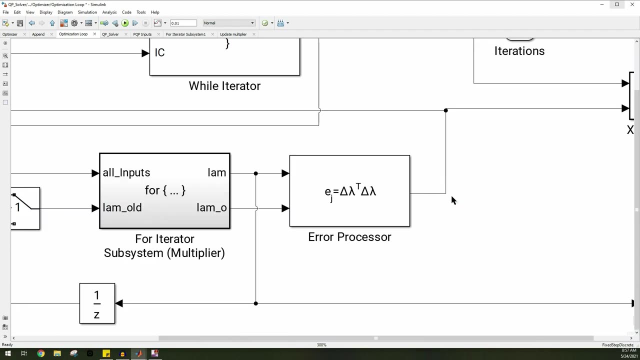 very important to know and that is why i have it there. so, with that being said, you can solve for the error. so this is simply lambda minus lambda old. that is my delta lambda transpose times delta lambda. so this is a simple multiplication and then i will pass the error into here. i check that the error is. 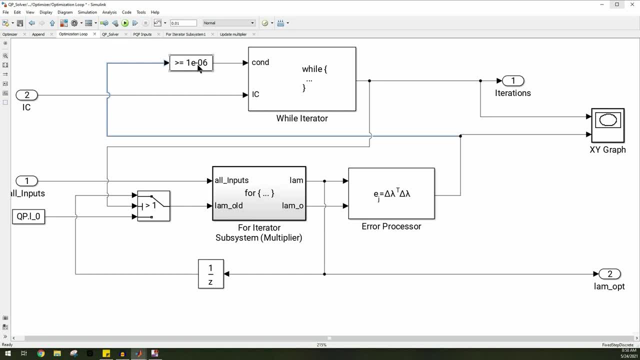 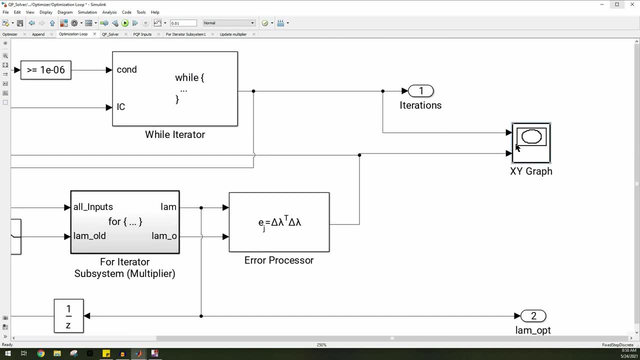 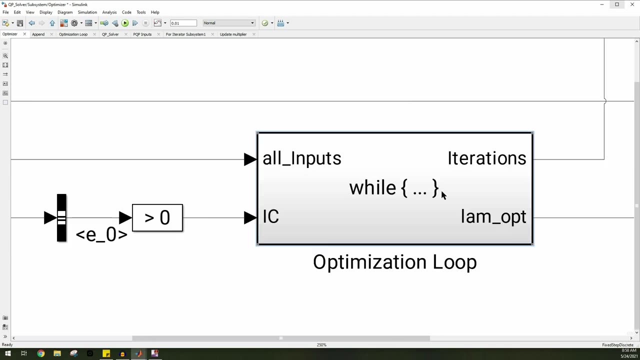 less than one to the power of negative six. if that is true, this iteration will stop. you can also output the iterations and the error like so in this x y graph there. so when i have my optimal lagrange multiplier, which is the output of this y loop and for loop inside it, i can then solve for. 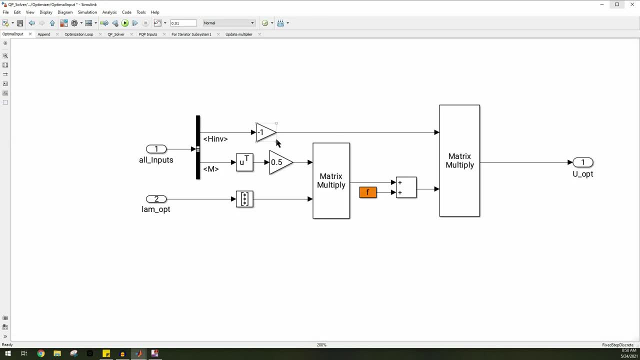 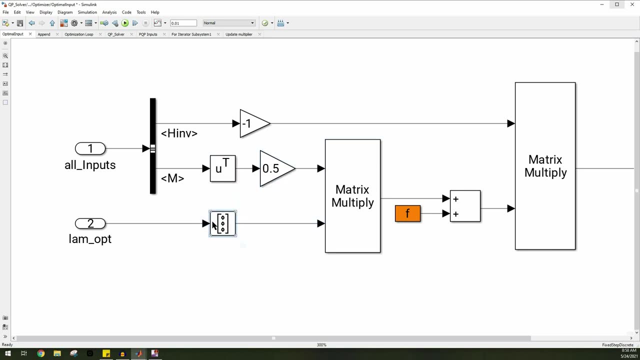 my optimal input. so this one is quite straightforward, so i'm just going to go ahead and do that and then move forward. you just simply do some basic math here, so just do transpose times, multiply times 0.5. you have to reshape this into a 4 by 1, so you have to make it a column vector because it is a column. 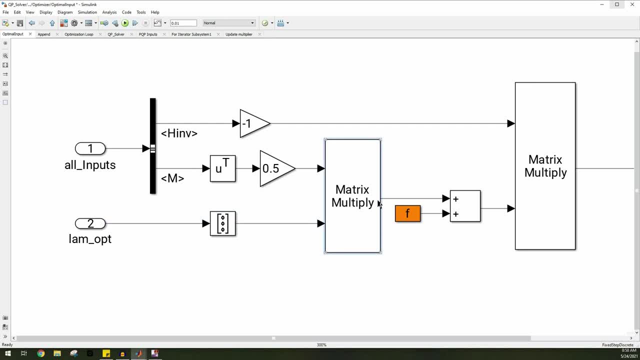 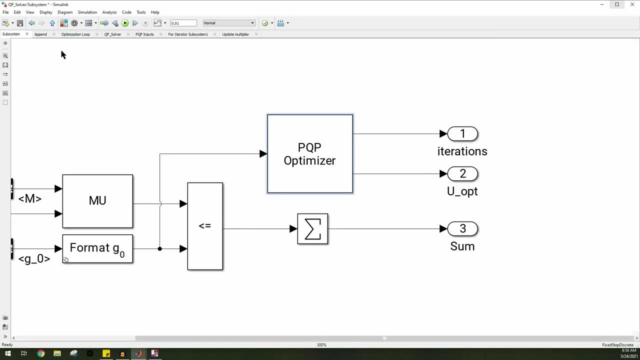 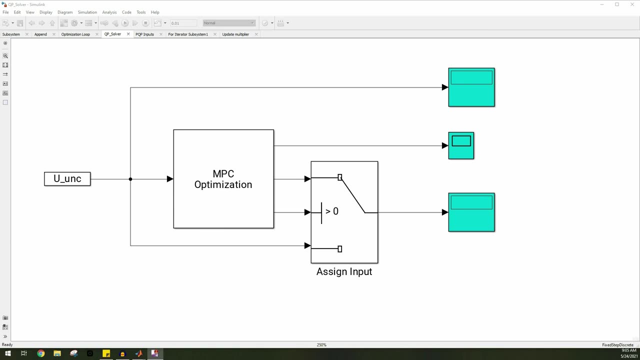 vector. so you will need this block- here it's called a reshape- and then you just add it to f and then you multiply it once again and then you get your optimal inputs there. so that's it for the program, and then let's see how it now, how it works. so let's run this model and see what we get. 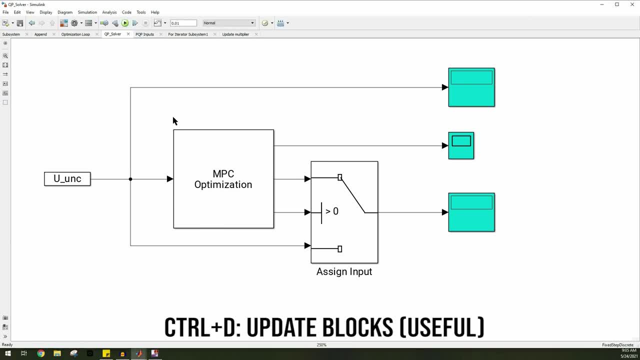 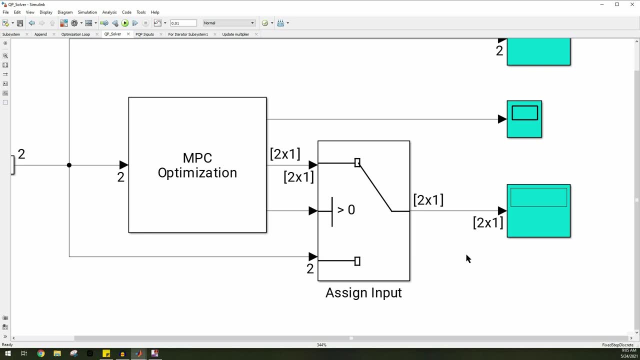 so if i go on first, you can do ctrl d to just update the blocks and you will see how you will get the signal dimensions there. so that's very useful. if i just press run now you will see the output. so this x- y graph is the optimizer. you can see how it the error goes to zero eventually. 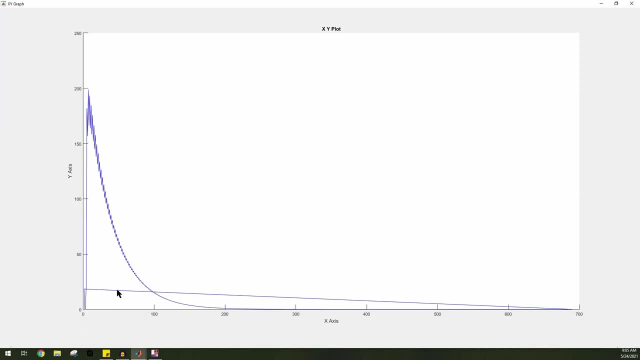 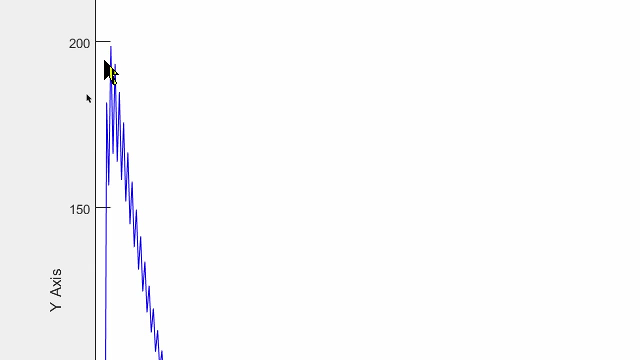 um, ignore this line here, the this one here, because it's just a bug. but it starts off at one. it goes all the way up to about 200, but then it'll come back down very fast and then it eventually goes to zero. you can see how it it solves for my input. so this is here is my unconstrained input. 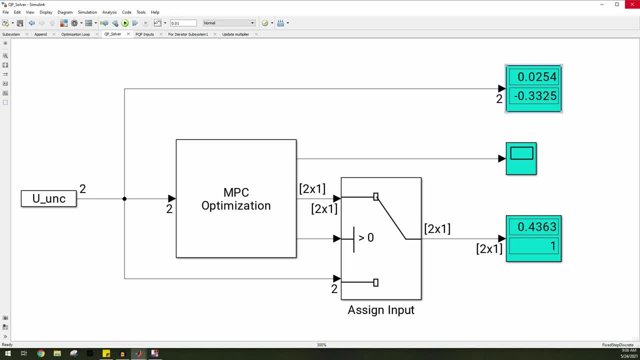 the bottom one does not meet the constraints because it is less than negative 0.15. but if i optimize this whole thing, it'll give you the constrained input. so it capped at one, which is the maximum value, and then 0.44. so this means that the optimizer does a good job of solving for these inputs. 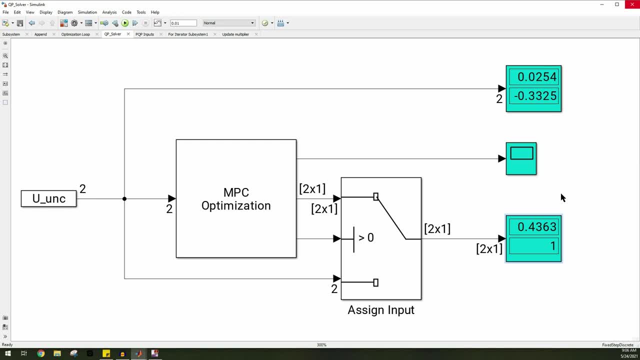 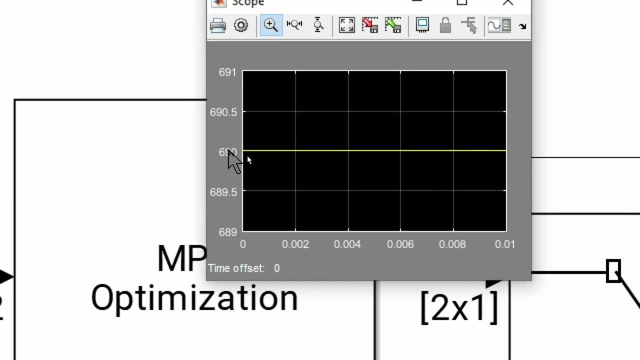 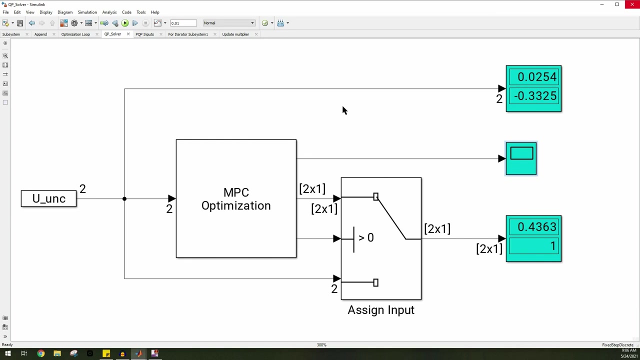 if i look at the scope, this scope here shows you the number of iterations which i used. it is about 700 if i auto scale this so you can see how it's about 690. so it took that many iterations for the optimizer to converge. so, that being said, i had this program works and it works well. thank you for watching you. 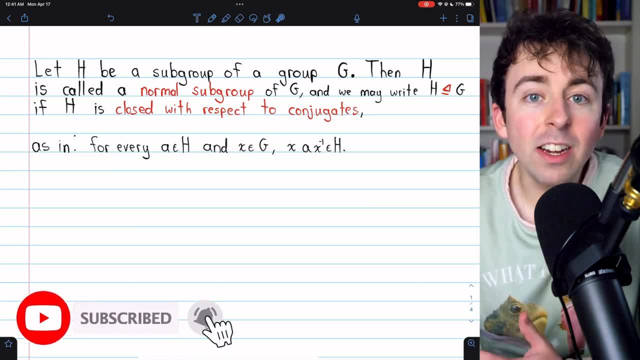 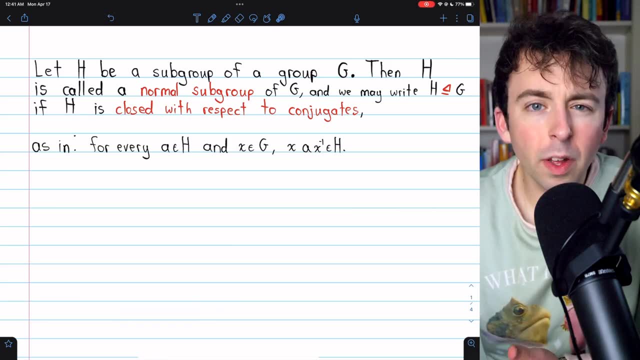 We're going to go over two equivalent definitions of a normal subgroup, then we'll see an example, then a non-example, and then we'll finish off with a quick proof of a basic result concerning normal subgroups. In later lessons, we'll see that normal subgroups are extremely important, 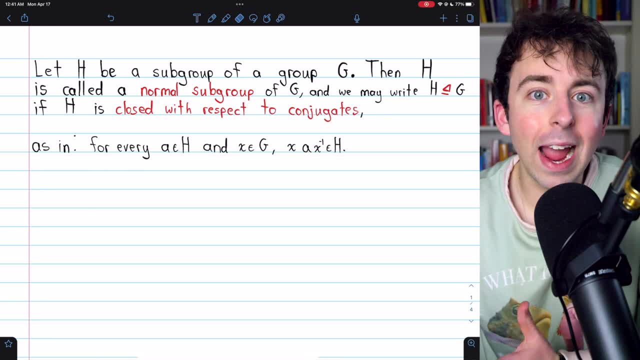 but for now, let's just focus on making sure we understand what a normal subgroup is. 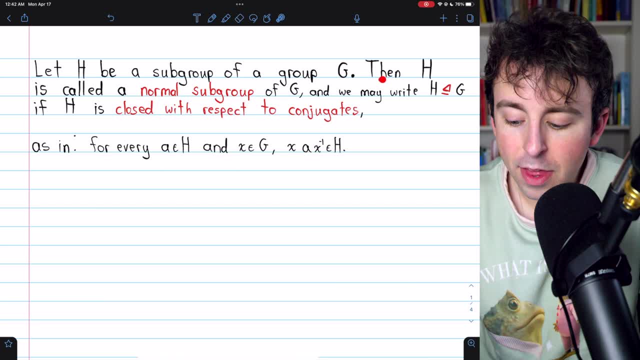 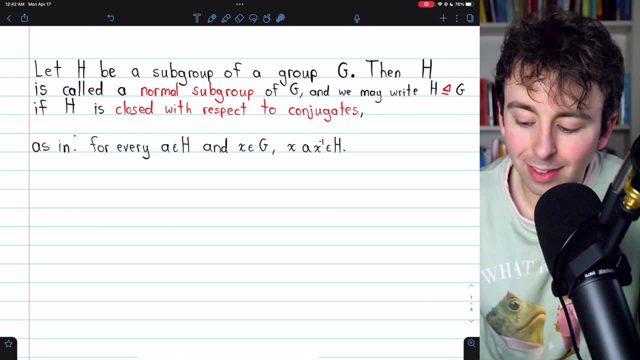 Let H be a subgroup of a group G. Then, H is called a normal subgroup of G, and we may write that like this, using a symbol that's like the less than or equal to symbol, but with a triangle instead of a less than. We may write H as a normal subgroup of G like that. If H is closed with respect to conjugates, the conjugate of an element A is any element of the form X, A,